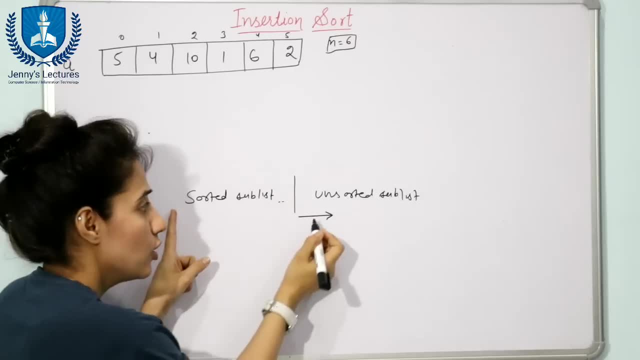 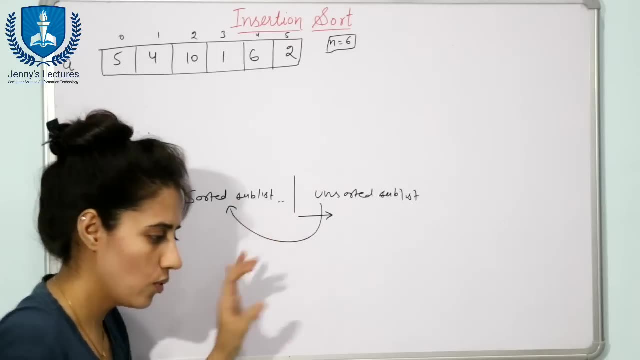 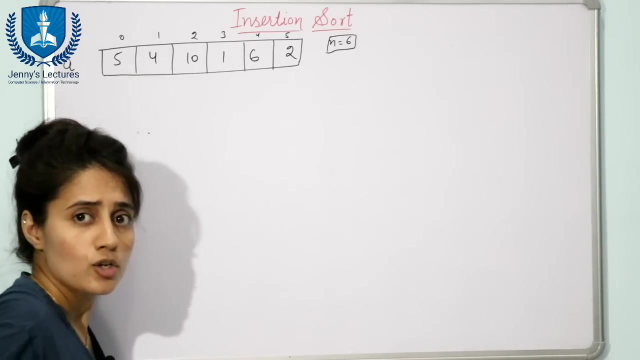 the appropriate place for that value in sorted sublist. We will insert that value in sorted sublist one by one. Fine, Now how this technique works. See first of all this: this is an array, or you can say: this is our list. Fine, So by default we are going to take: see this first variable. 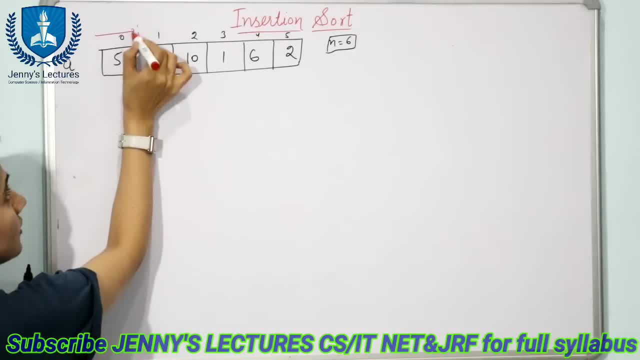 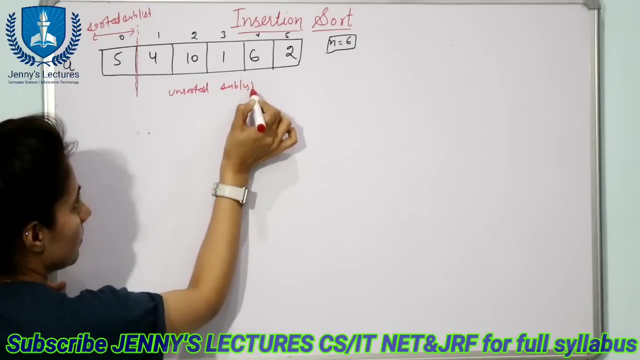 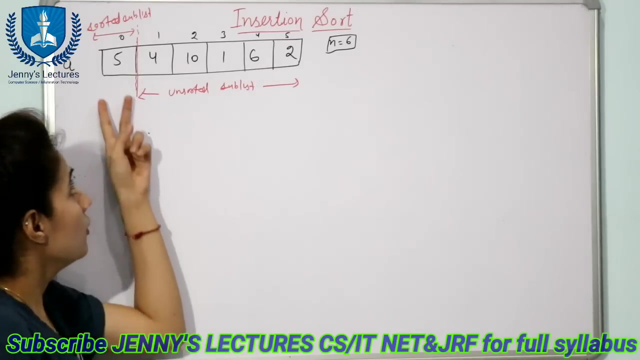 This is note appears One score pair. This is we are going to consider hazard Sorted Sublist. And from index one to the last, This is a And sorted sublist. See, while you're going to take one variable in sorted sublist, 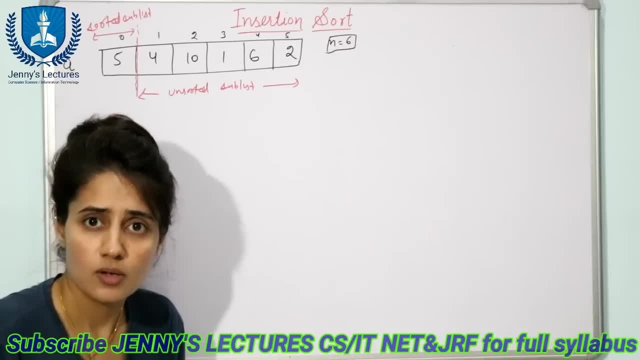 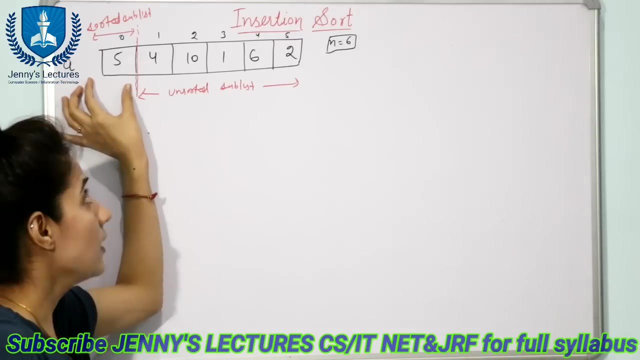 having one value, then that value is always sorted, because only one value. you have no need to compare with any other values, so that value is always sorted. so by default, we take what this, a of zero, this value is sorted and we are going to start our loop from here only so. this is unsorted sublist. 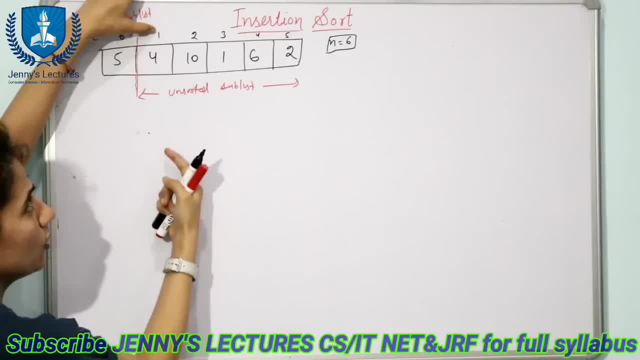 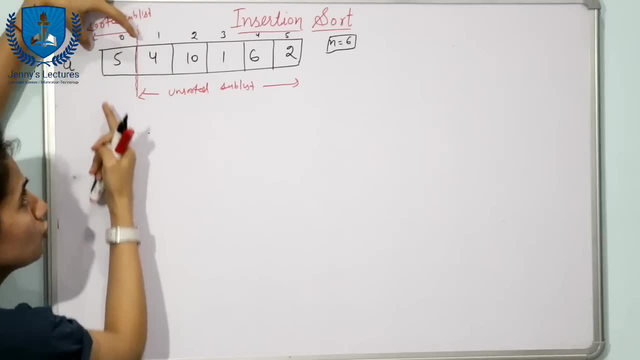 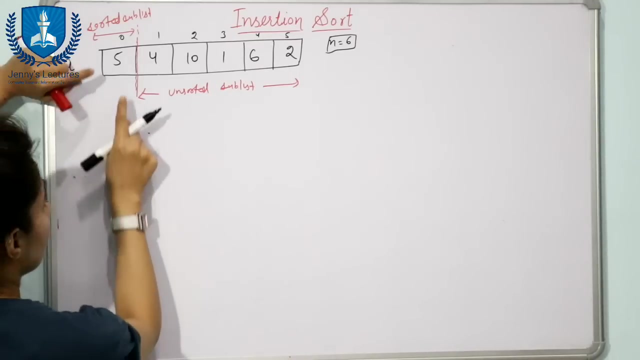 we are going to trace this unsorted sublist starting from here. only one by one, we take values from unsorted sublist and we are going to find the appropriate place for that value in sorted sublist and then we are going to insert the value in sorted sublist. fine, now see, first of all: 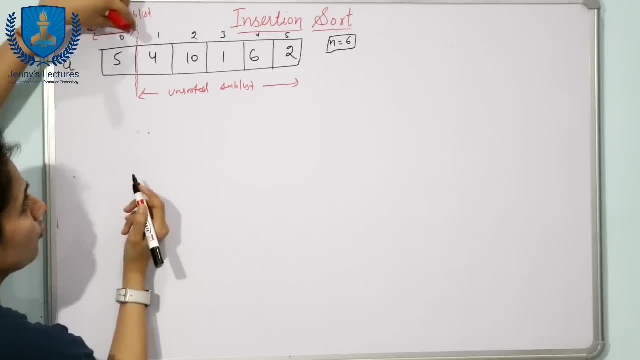 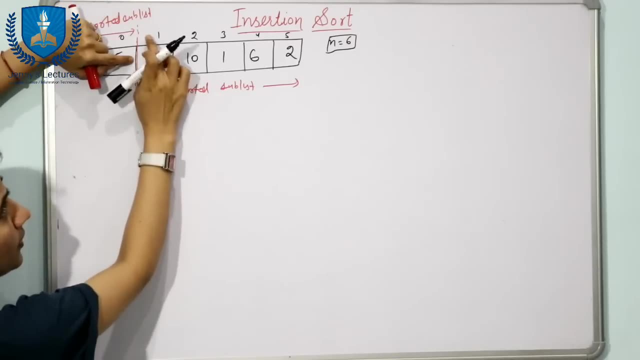 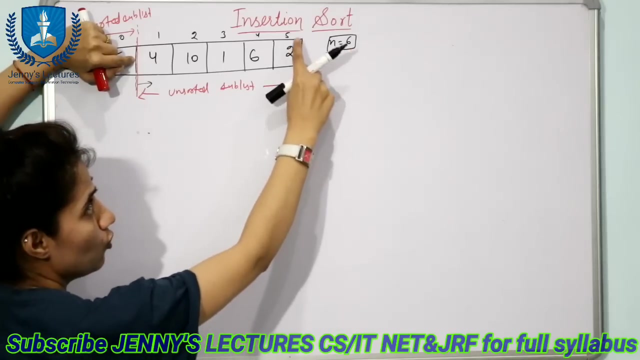 this is our sorted sublist. this is unsorted sublist. now we are going to start from here. we are going to trace out this unsorted sublist from starting. so starting of unsorted sublist is from index 1, so the loop would be from 1 to n, less than n. n is 6, so loop. 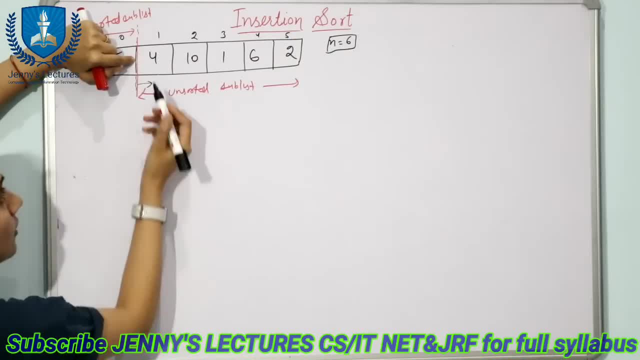 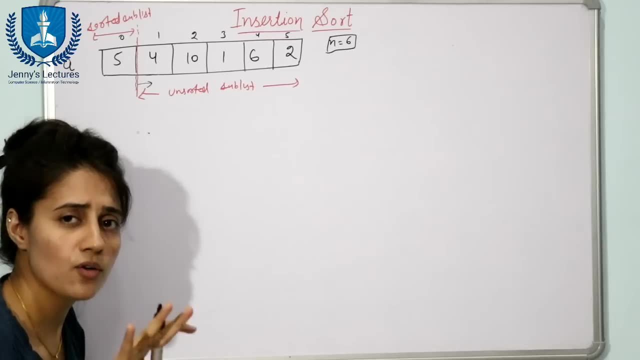 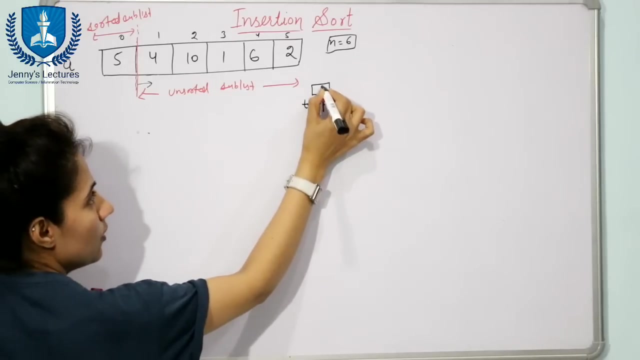 would be from 1 to 5. okay, now see, first of all, take this value, this value 4, and when we are going to take this value, then this value is to be stored in a variable, suppose temp. we are going to take one variable, temp, and we are going to store this value 4 in this temp variable. now we have stored 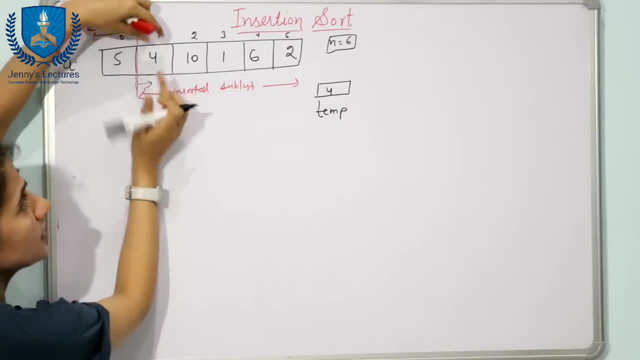 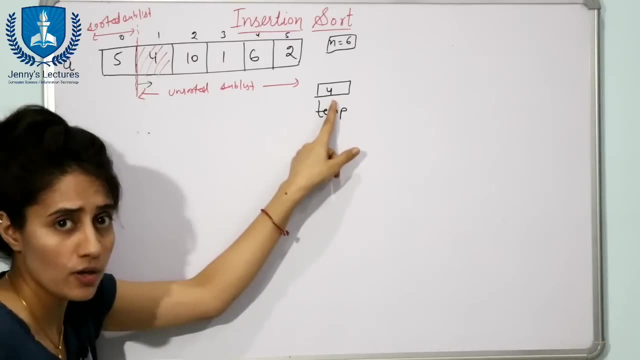 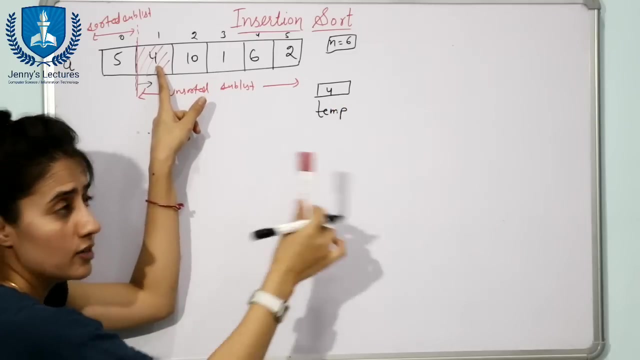 this, this value in temp variable. now this: this is considered as a whole. actually, we have copied this value here only so we can overwrite this 4 in this array now, because we have backup of this value. in future if we need this value, then we can use this temp variable. so this: this is considered. 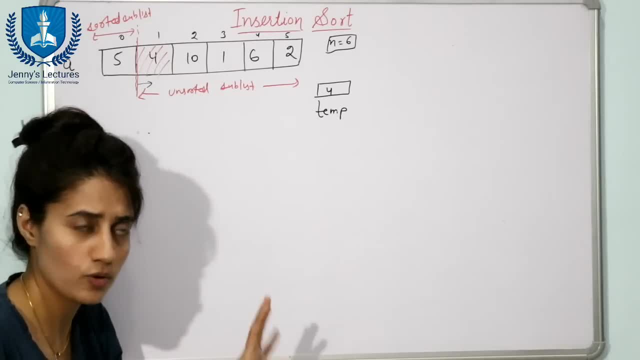 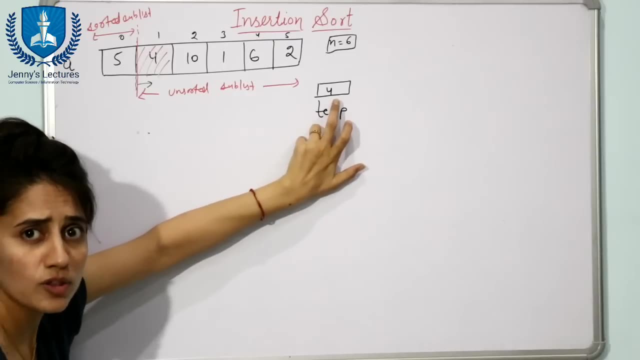 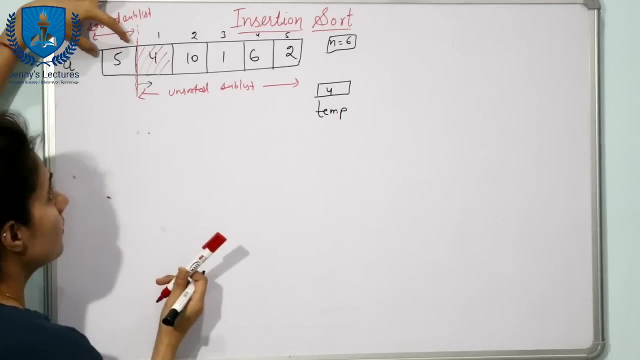 as a whole now find free space. you can say you can overwrite this space here, only now. second step is this variable is to be compared with the variables in sorted sublist. we are going to find out the proper place for this variable in sorted sublist now. in sorted sublist we have only one, one value, that is 5. so 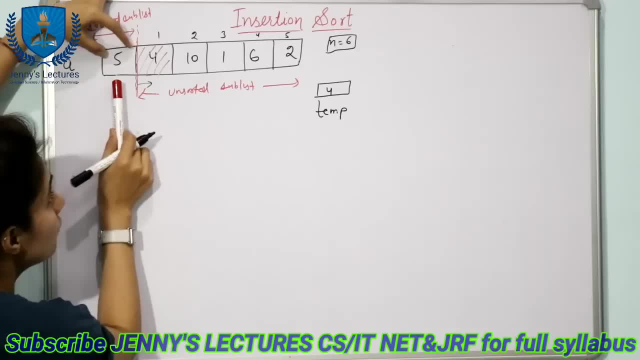 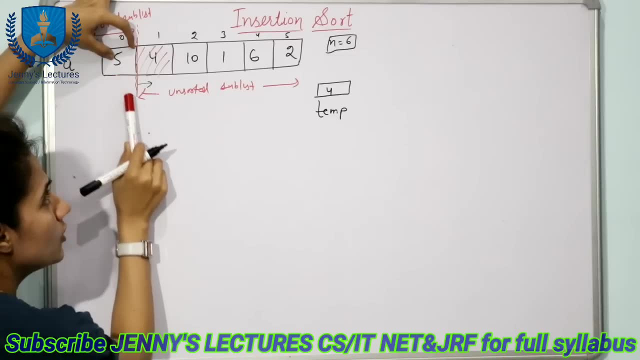 compare this 4 with this 5. now, if this value is, see, this value is greater than this temp value, then what you will do? then you will shift this value to its right position by 1, see, by 1. so now, here, 5 is greater than this 4. 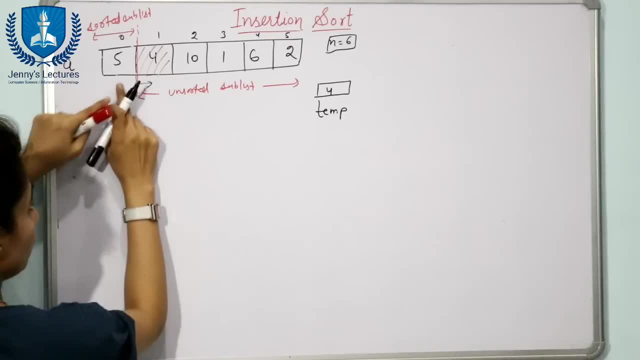 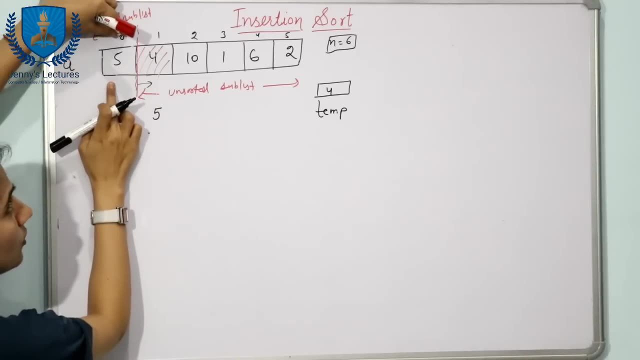 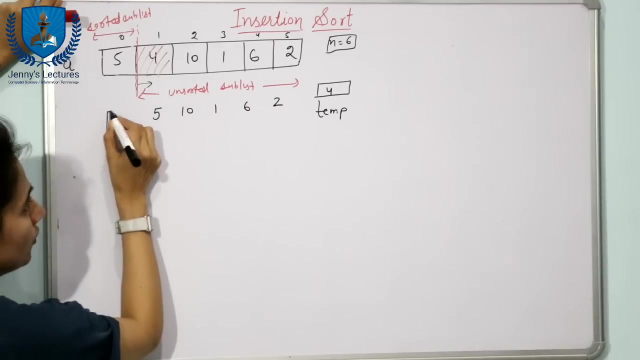 yes, now what to do now? this 5 would be shifted one place right, so 5 would be now here. only 5 is at place a of 0. now 5 would be at place a of 1. now the array is 10, 1, 6 and 2. fine. 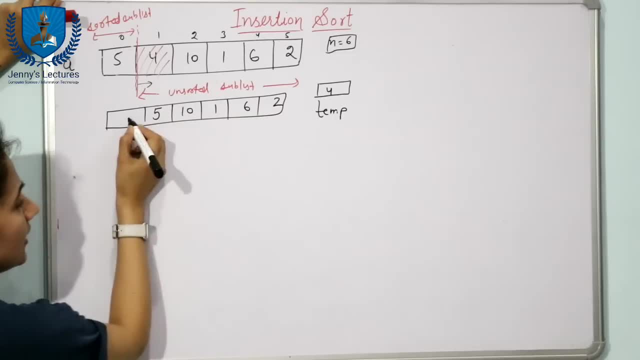 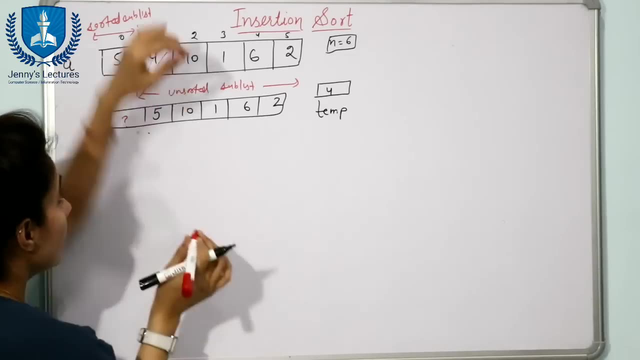 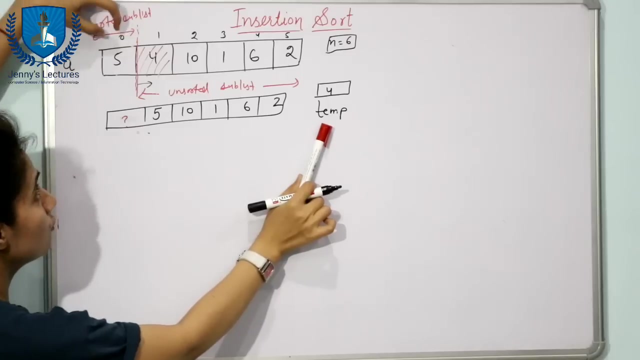 now at this place. it's not like we directly directly put 4 here. no, still it is a question mark. now, is there an any other value in sorted sub list which with which you can compare this temp value? no, because we have reached to index 0, so there is no other value now. if there is no other value, then you can put. 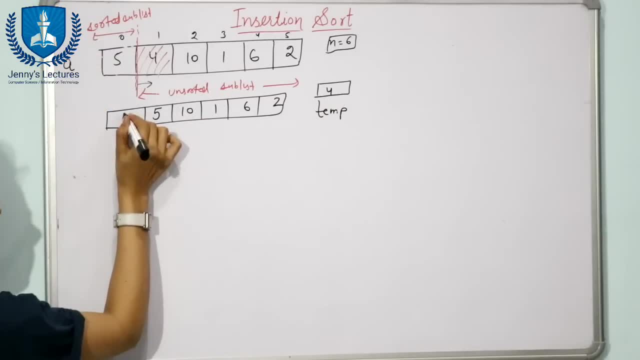 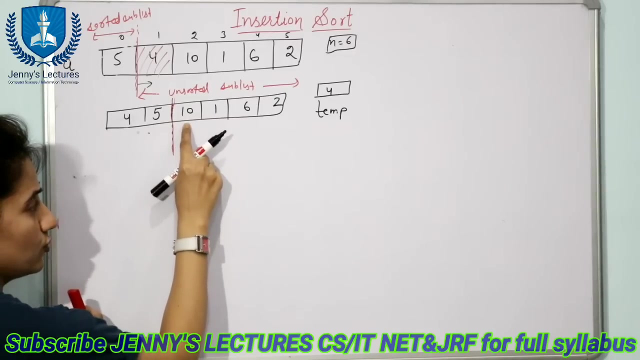 this 4 at this free space now, 4 would be here only fine. now sorted sub list. is this one? now, this is our sorted sub list and this is now our unsorted sub list. so now again, we are going to take the first variable from unsorted sub list. we are going to store this variable in temp now. 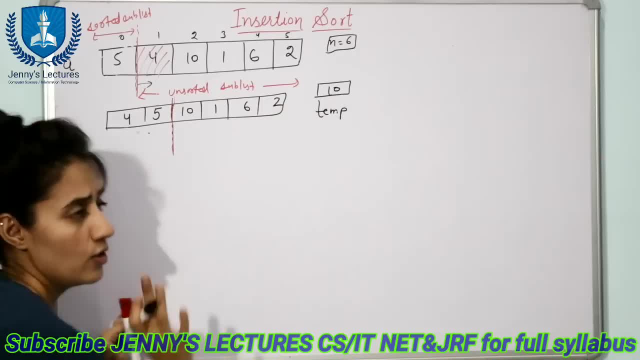 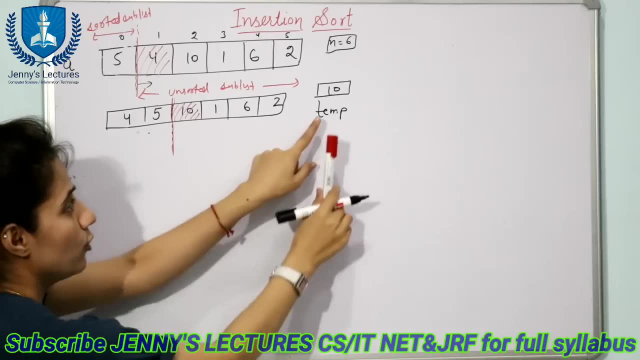 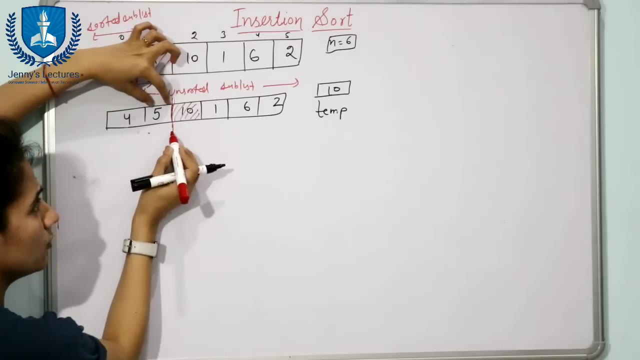 here temp value is 10, now temp value is 10 and this is considered as a whole. now, now same second step is we are going to compare this temp value from with all the values in sorted sub list. we are going to start from here. only we are, we are. we will move from right to left in this sorted 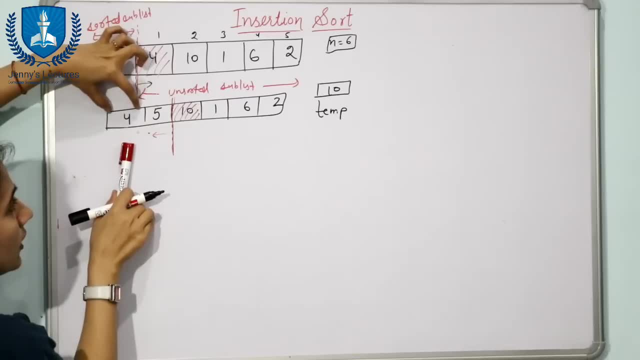 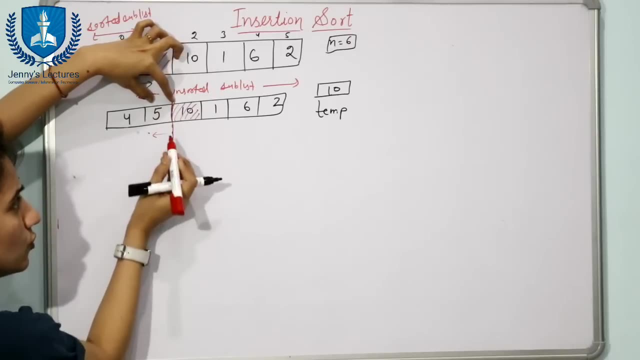 sub list. it is not like in sorted sub list. we are going to take first of all the 0th index. we are going to compare with the 4, then 5. no, we are going to compare with this value first of all. we will move right to left till we reach. 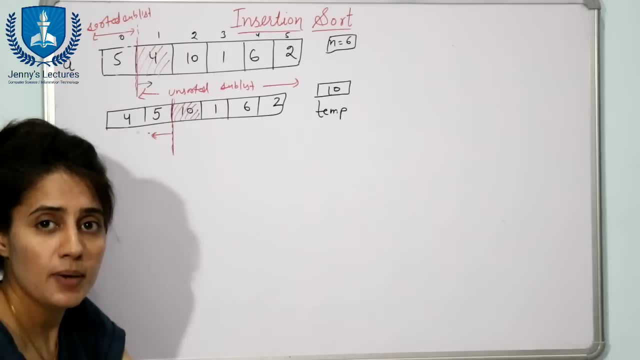 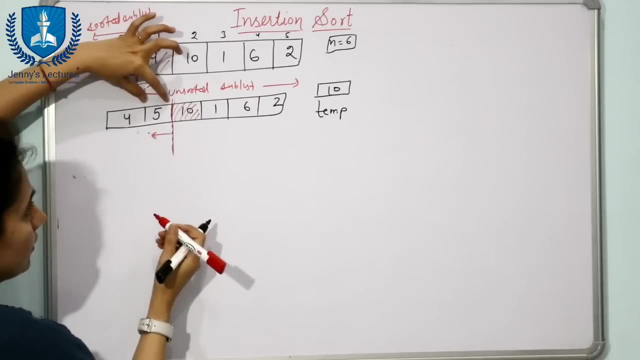 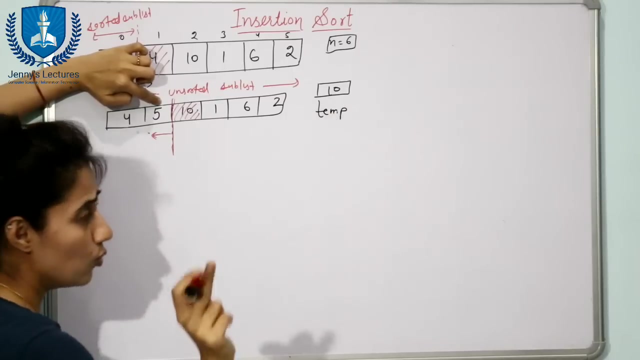 to 0th index. so this loop would be decremented by 1 and this loop would be incremented by 1. two loops would be there. fine, now see first 5 value. then 5 would be compared with temp value. is 5 greater than this temp value? no, fine, then no need to right shift this value. simply if this: 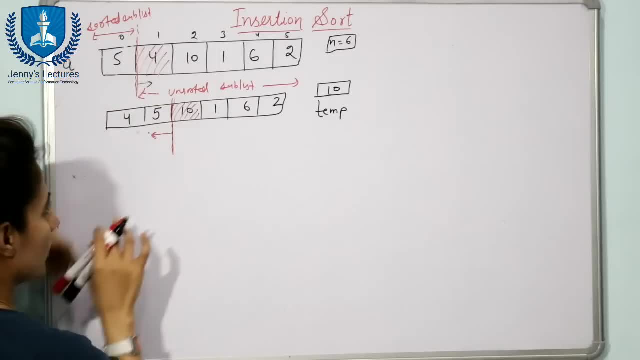 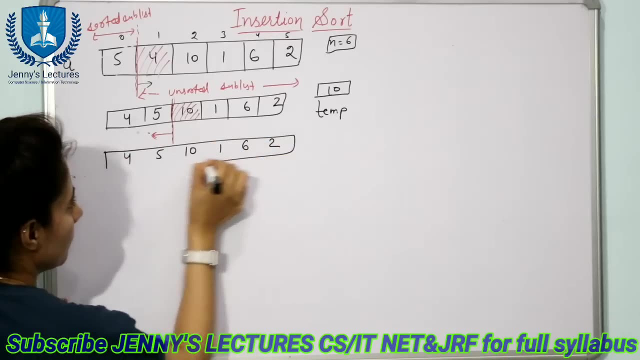 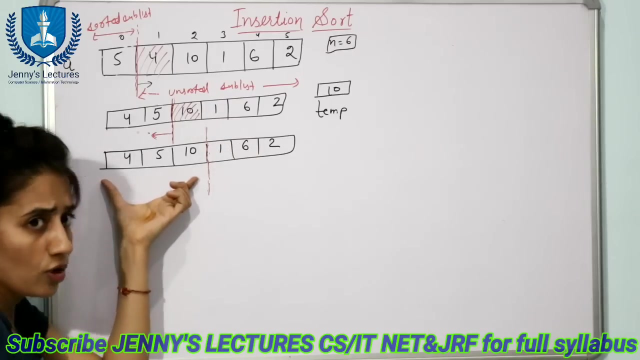 condition is not true, then simply you will insert 10 here only, and the array would be something like this: 4, 5, 10, 1, 6 and 2. now, this is the sorted sublist. now, this is now sorted sublist, and this is now your unsorted. 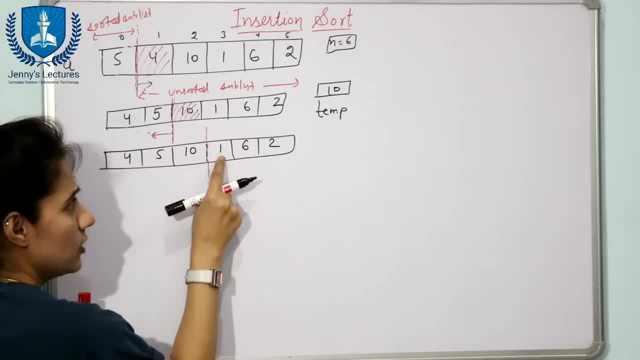 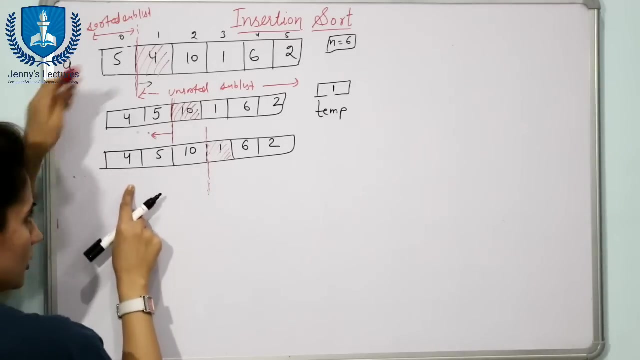 sublist. now take first variable from unsorted sublist: 1 we are going to take, and in temp we are going to store now 1 and this would be considered as a whole. now, fine. now second step is compare with the values in unsorted sublist. now we are going to start from here only. 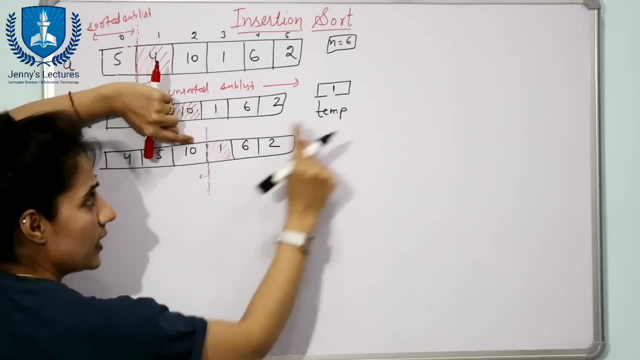 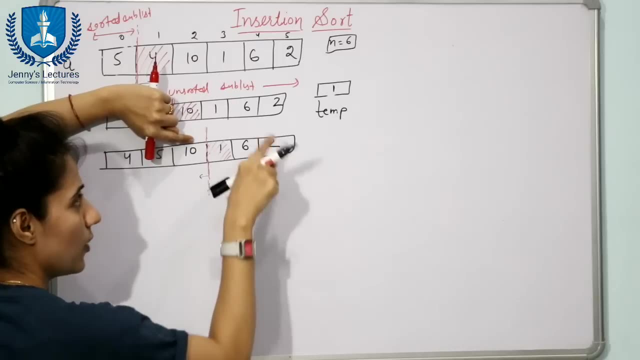 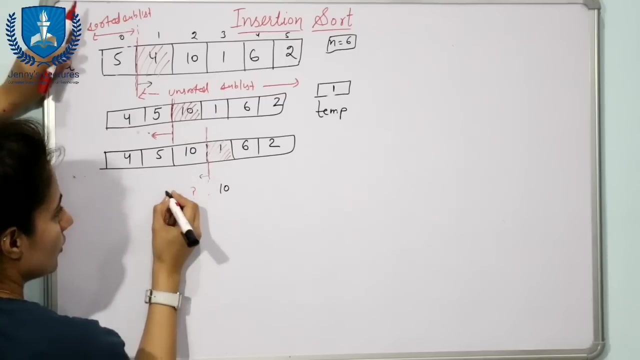 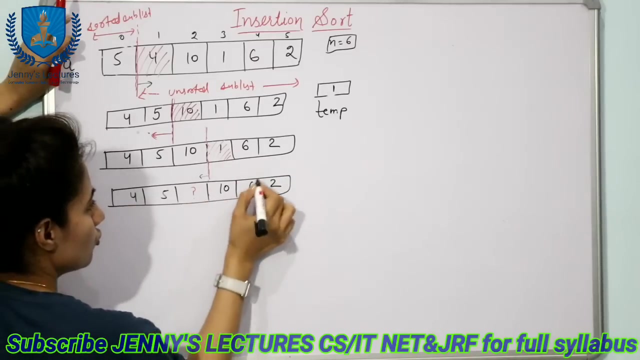 first value is 10. is 10 greater than this temp value? yes, if yes, then we are going to shift this value one bit right. so 10 would be shifted at this place. now. here question mark: now here we have four. five, here we have four. here we have six. here we have two. it's not like that you directly store now. 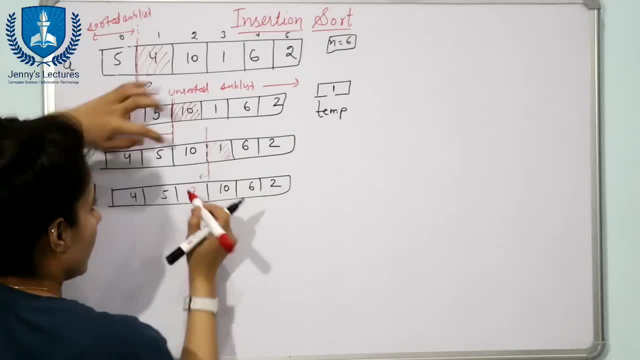 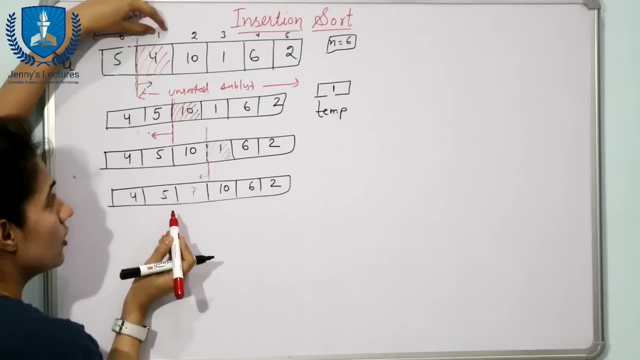 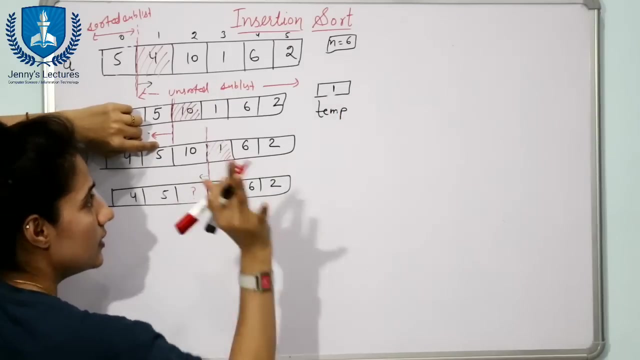 one here. no, still, we are not going to store here again. next is this one. now, index value is two. now, if you decrement, then index value would be one. now, this value five. this five would, be compared with this, one is five greater than one. yes, then again, five would. 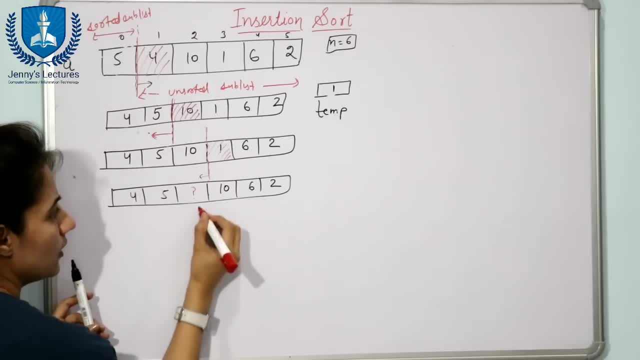 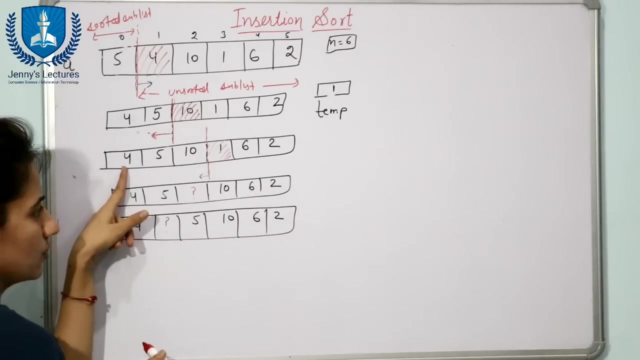 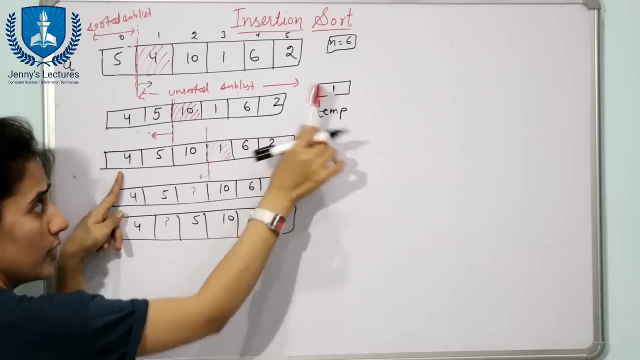 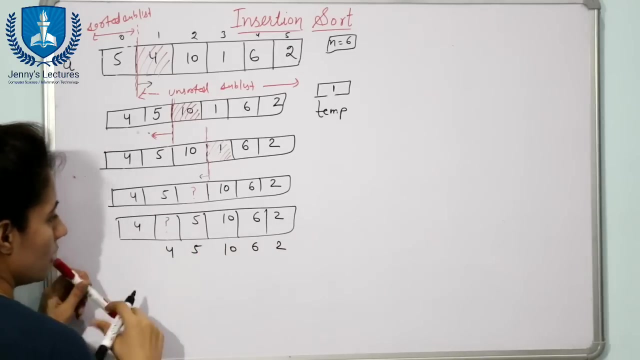 be shifted one place right. so five would be shifted here. only so five, ten, six and two. now here is question mark. here we have four. next, compare with this: now four we have compared to five. now with four, is four greater than this temp value? temp value is one. yes, again, shift four at right place. now four would be here, then five, ten, six and 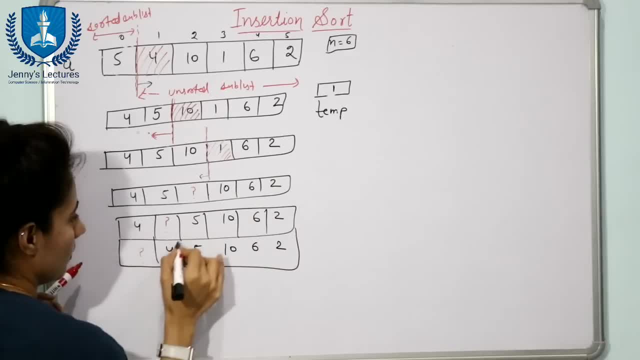 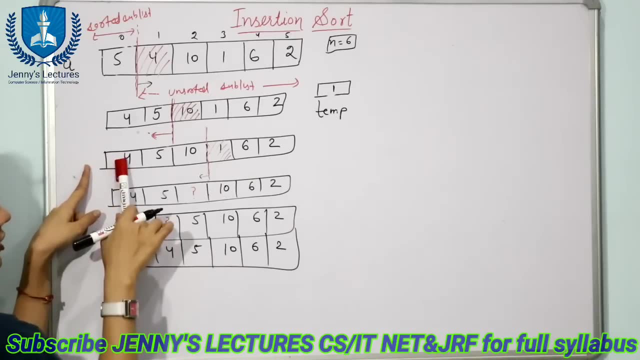 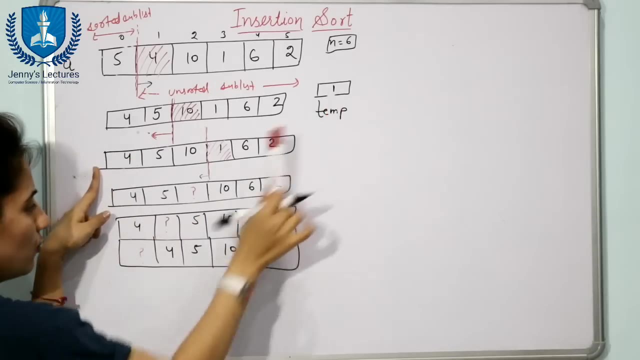 here is question mark. now is there any other value in sorted sublist left? no, we have reached to index zero, so now we cannot compare now with this temp value with any other value. fine, now we just insert this temp value here, when now one would be inserted now. 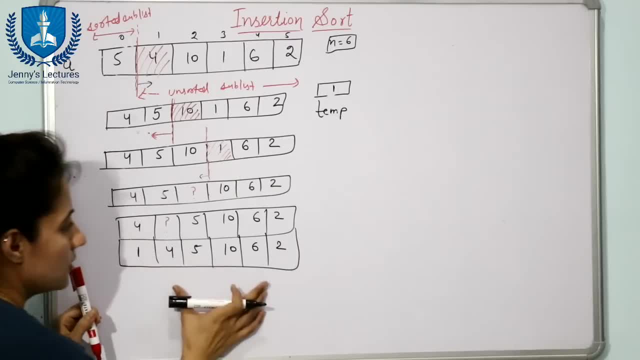 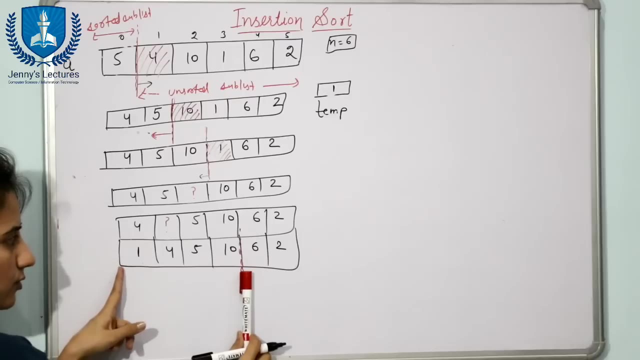 here at last. fine, now array. is this one now sorted sublist? is this is now in sorted sublist here. we have three elements now here after sorting, after after inserting this one here, four elements are in sorted sublist and two elements are in unsorted sublist. now we are: 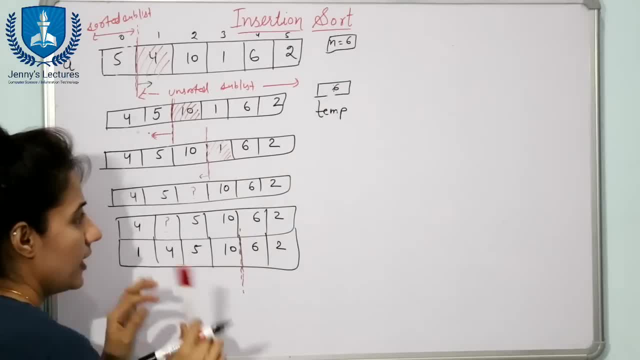 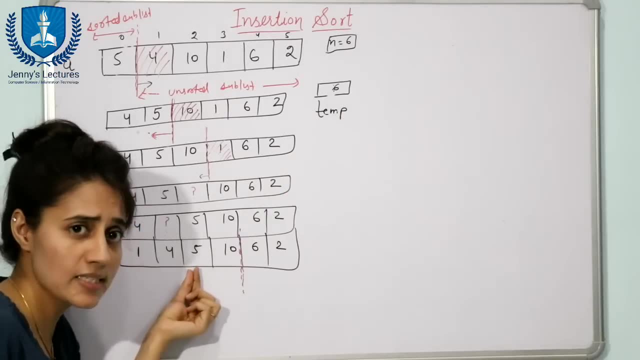 going to take this six we are going to store in temp and now we are going to compare with this six, with these values, to find out its appropriate place. and once you find out the proper place for this six, then you just insert this six here. only it's not like you all, you have to compare the six. 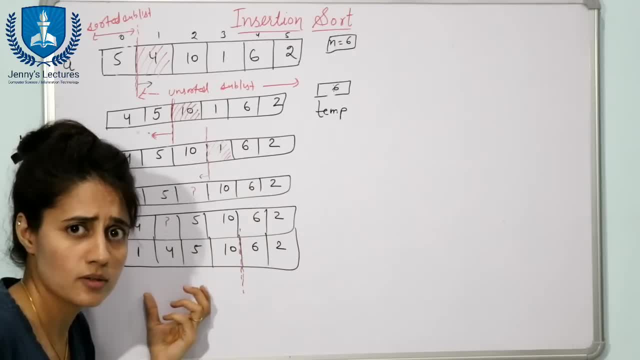 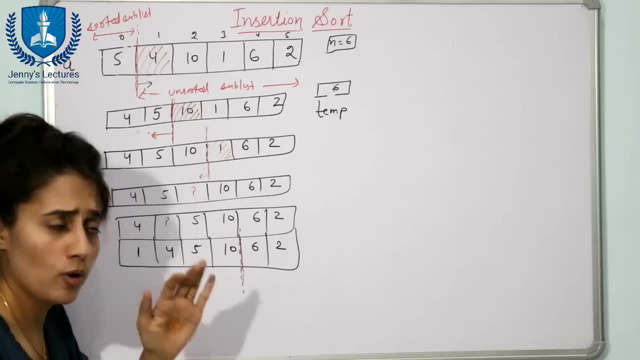 with all the values. no, just find out proper place. as soon as you find out the proper place, you just insert this temp value. fine, if you are not finding out the proper place, like in case of one, then obviously we have compared this one with all the values. and because at starting 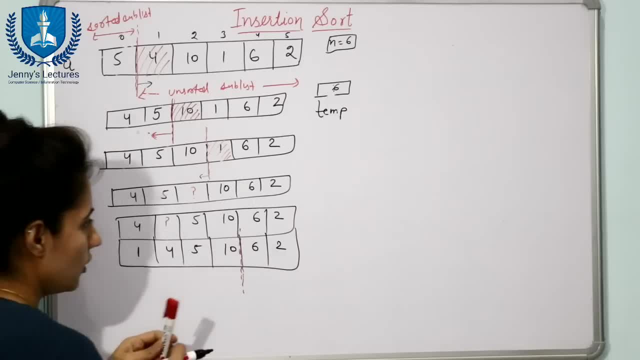 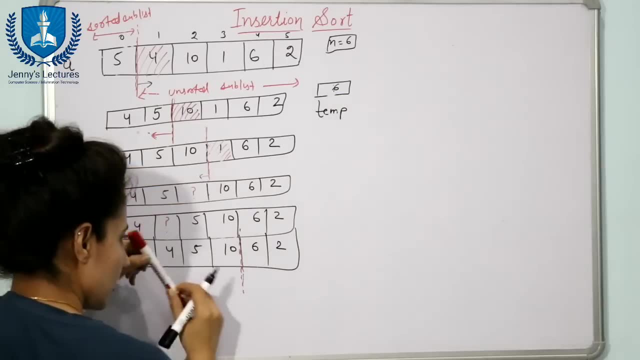 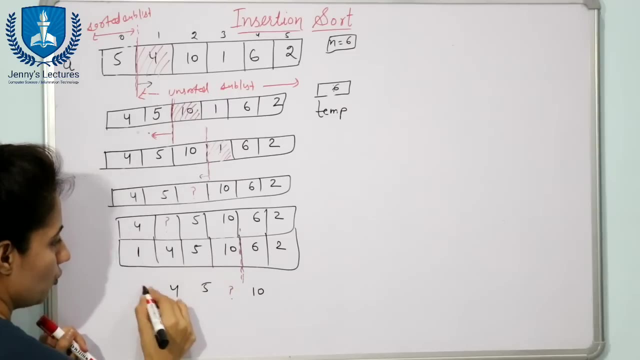 only we can insert this one. fine now in case of six. first of all, compare with this: ten is ten greater than six? yes, now we are going to shift this ten one place right. so now ten would be here. only here is question mark. here five, four, one, and here we have two right next. next value is: 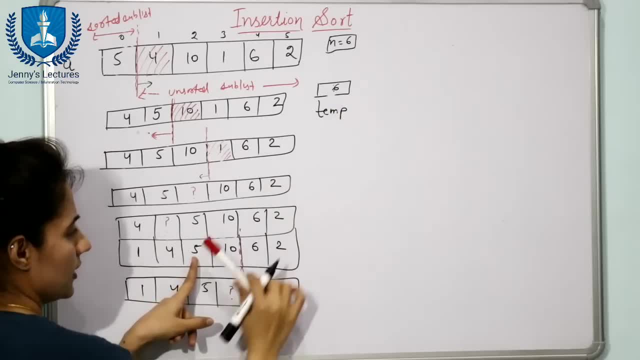 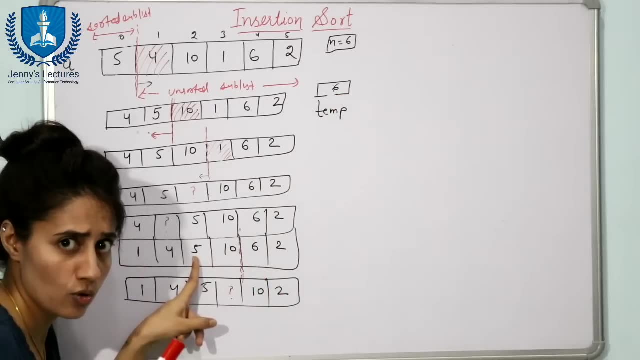 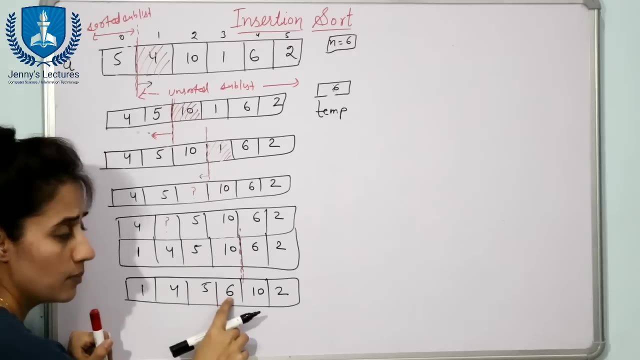 five. we will compare this five with six. is five this value greater than this temp value? no, then no right shift would be there if condition is not true. fine, now, simply you insert this six here, and obviously this is the proper place for the six after five. now this is our sorted sublist. 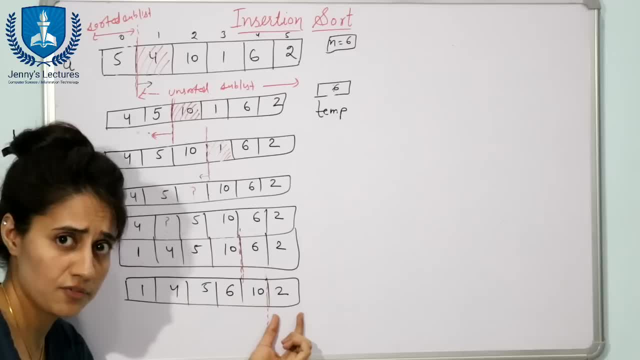 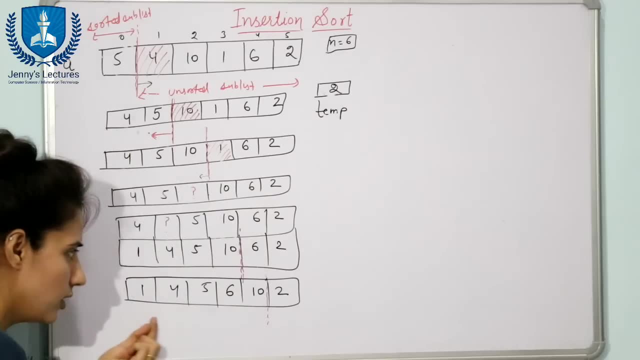 and this is our unsorted sublist. only we have one element left. now we take this, this value, we are going to store this two in temp variable and we are going to compare with this sorted sublist to find out the proper place for this six. and this is our sorted sublist and this is our unsorted sublist. 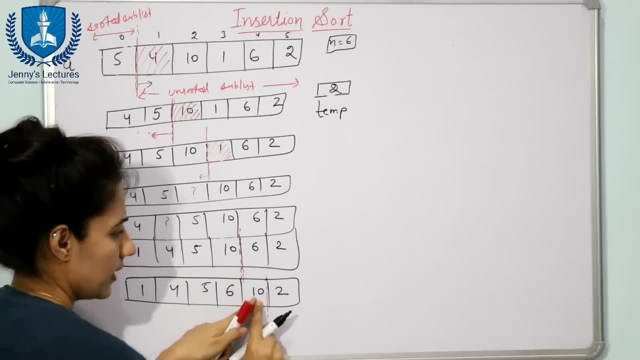 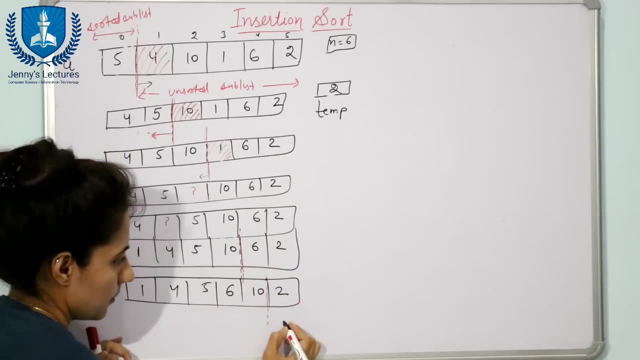 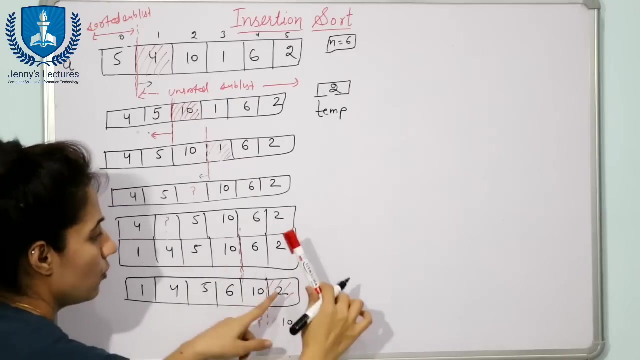 for this two. first of all, compare with this: ten is ten greater than two temp value. yes, now we are going to shift right. shift this ten one, one step here. now, here we would write ten. here is question mark, because if we have, we have stored this two value in temp, then this is considered as 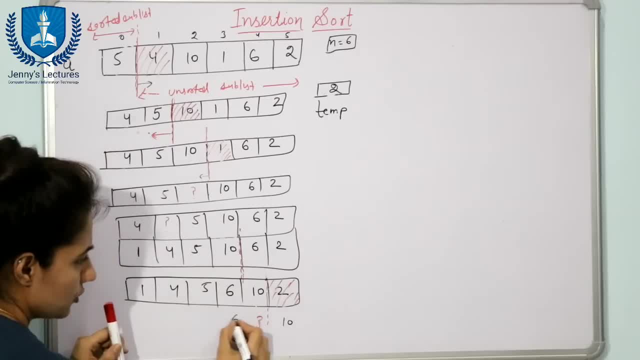 a whole. fine, here we have six, five, four and one. now again compare with the six, with ten we have. compared then with six. we compare: six is greater than two. yes, then right, shift this six. one place here now. six would be at this place now. here we. 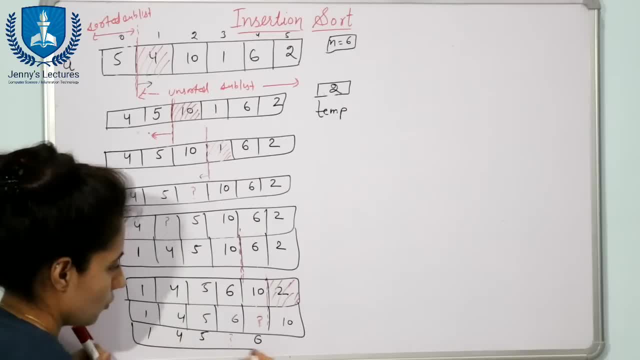 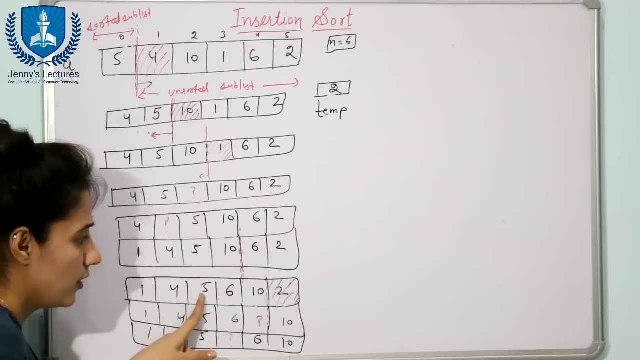 have question mark. here we have five, here we have four, here we have one and here we have ten. now we have compared with this six. now compare with this five. next value is five. five is greater than this two. yes, right, shift this five. one place this side. 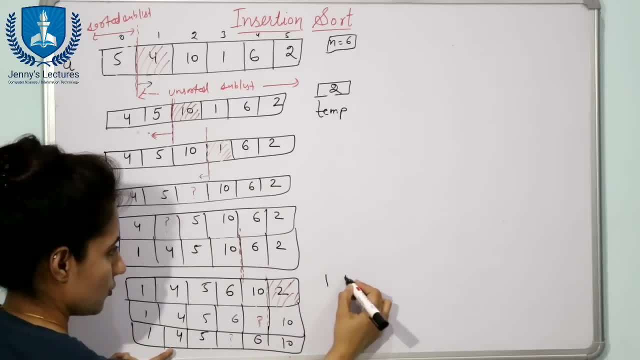 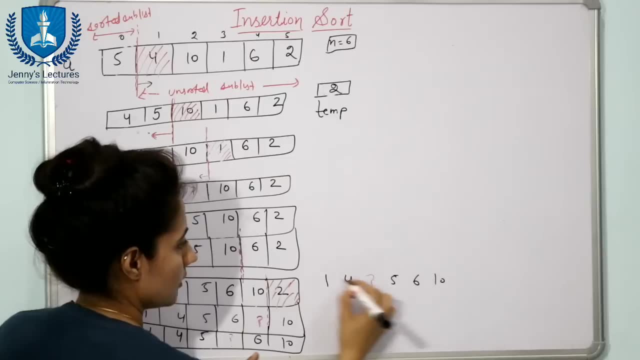 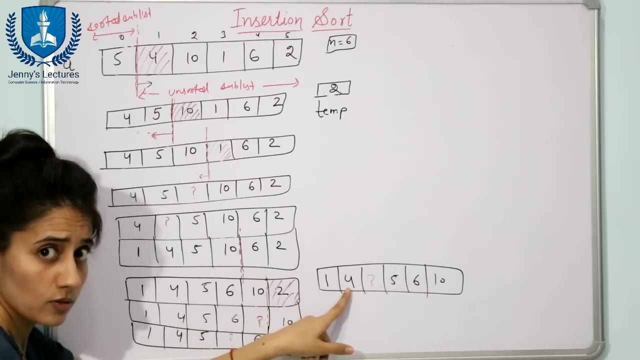 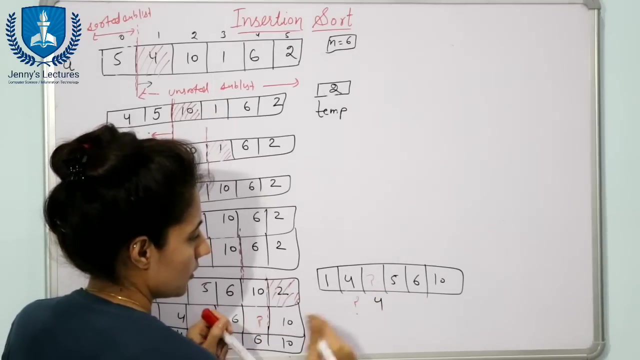 now the array would be: here we have one. four. here we would have question marks. this five would be shifted here. five. here we have six. here we have ten. now compare with this: four. fine, is four greater than two? yes, then right, shift this four one place. four is here now. here we have question mark here. 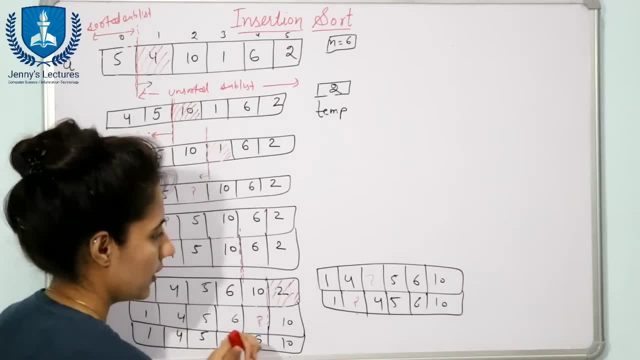 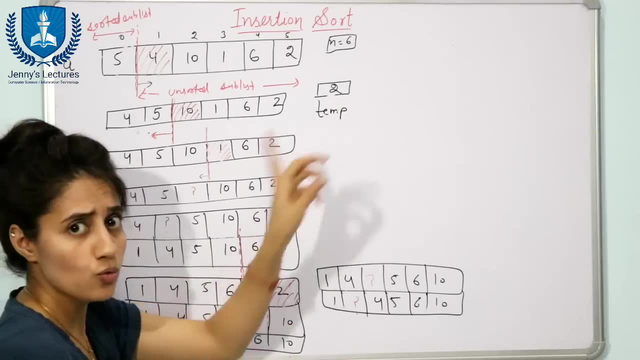 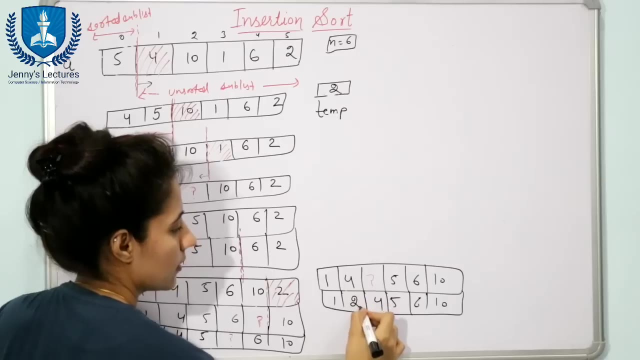 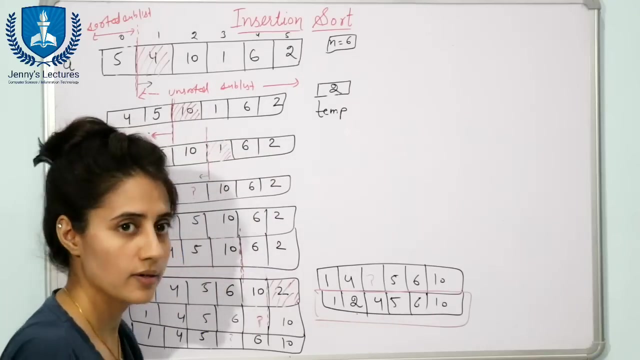 we have one now. this is the value. fine now. next is one. now compare with this: one: is one greater than this two? no, then no right shift would be there. we simply insert this two here and this is now our sorted array. you can see one, two, four, five, six and ten. so why this is no, why this is known as insertion sort. see, as you have seen. 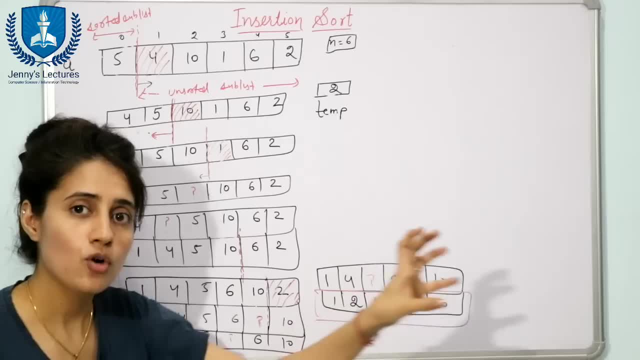 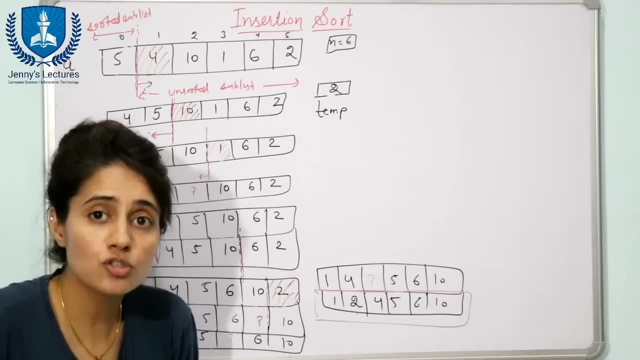 with this working principle. we have just taken one value from unsorted sublist and we have inserted that value in sorted sublist. that is why it is known as insertion sort. fine, now how to code this value. as you know, from here only, you can see two loops would. 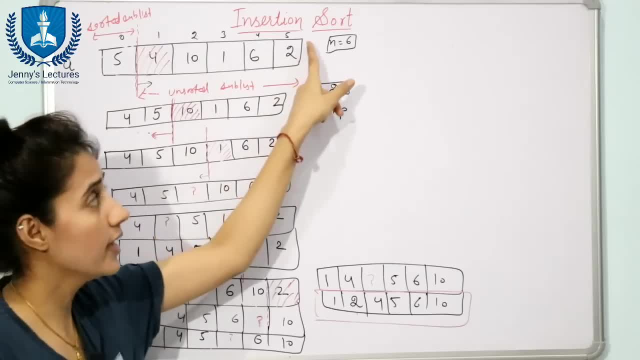 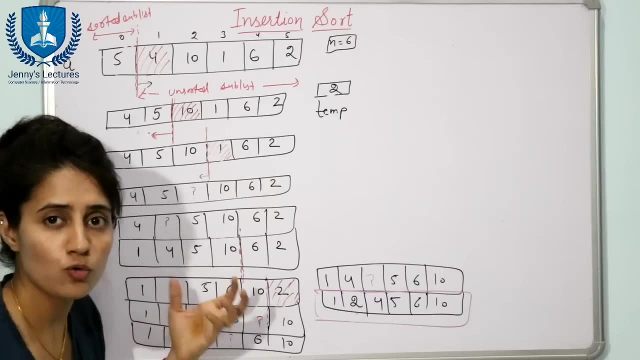 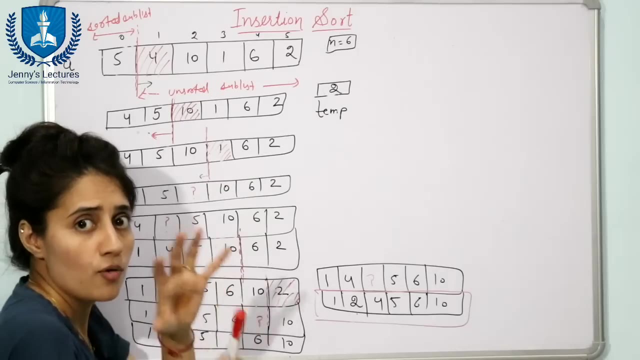 be required. one would be incremented from here to here and one would be decremented. why this decrement? because because of that comparison, we are going to find out the proper place for that element in sorted sublist. fine, so two loops would be there. so now the outer loop would be from here to here only because, first of all, we have taken this four and stored. 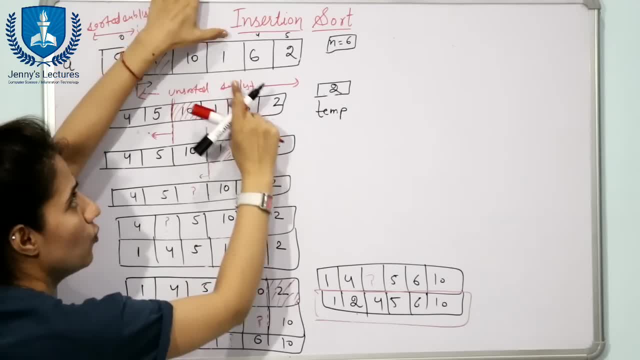 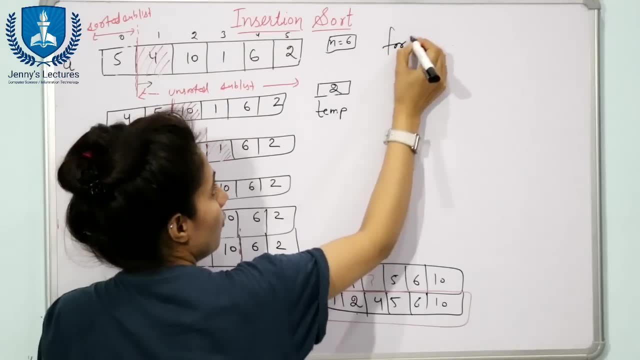 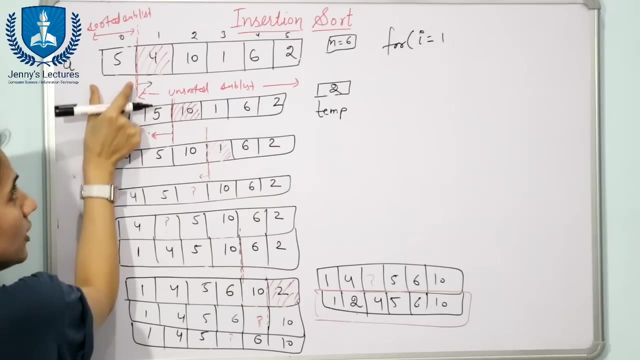 then temporarily in temp variable, then 10 we have taken, then we have taken one, then sixth and then two till we have, until we reach to the end of the array. fine, so outer loop would be: four, i is equal to one, i is equal to. we have started from one, because this is we have considered a of zero as 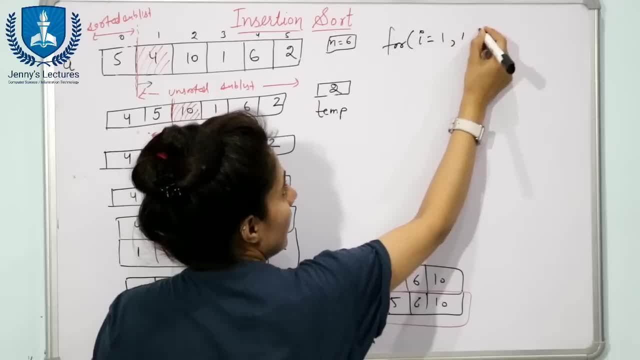 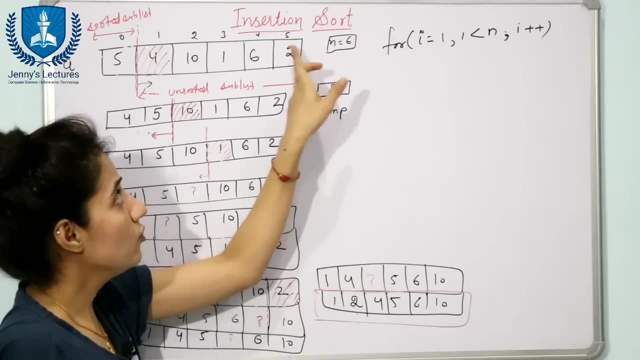 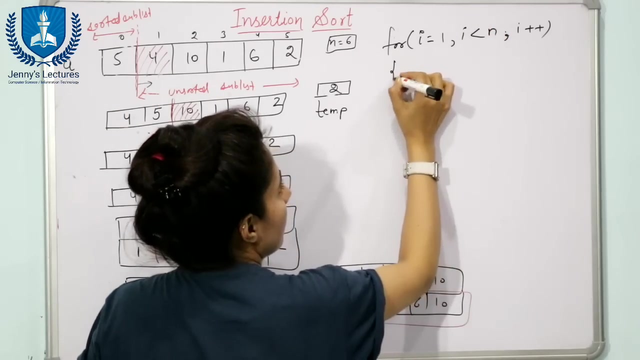 sorted sublist: fine, one, two less than n and i plus plus it is less than n, n is six and i value would be incremented to five, only index, because we have taken from zero, zero to five. so so now next step is. next step was: was what we have taken, this value? 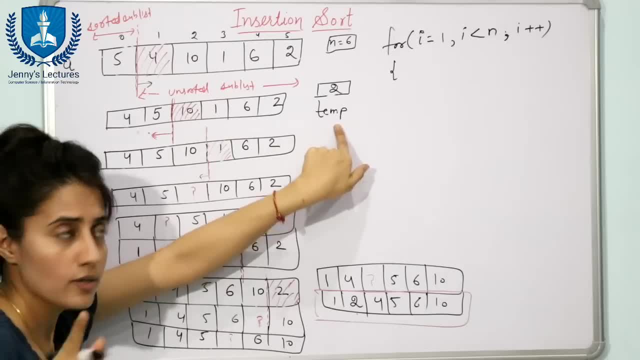 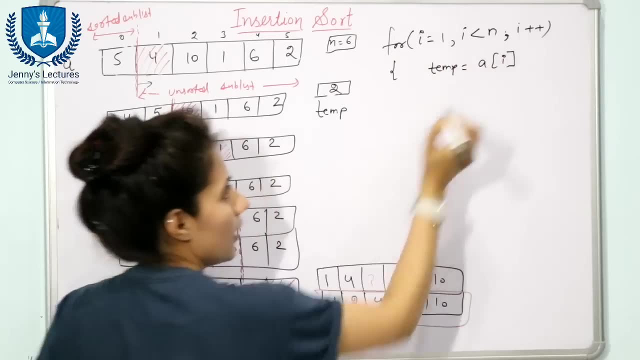 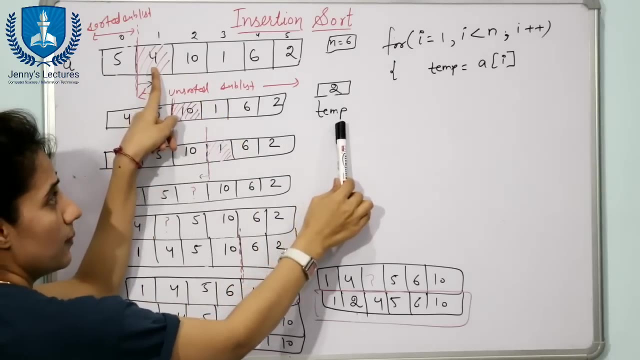 and we have stored that value in temp variable, right. so now next step is in temp variable we will store what a of i, a of, first of all i was one, and then we have taken this value and we have, then we have taken four variable, four, this value, four, and stored in temp. then i value would be. 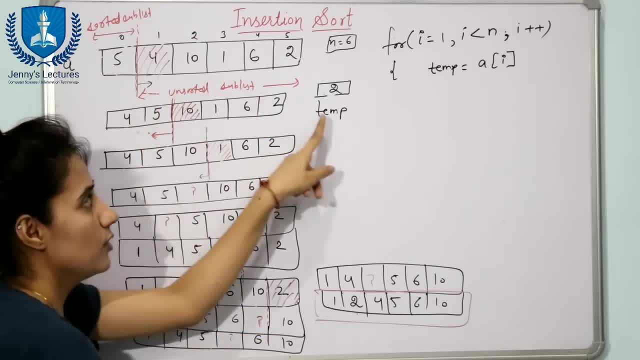 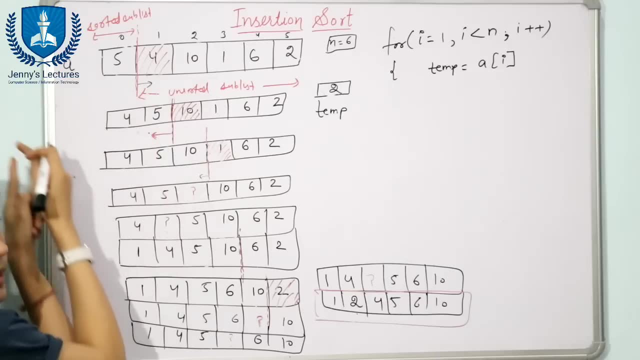 incremented. i is two. then we have taken a of two, that is ten, and we have stored in temp variable. fine, so temp is equal to a of i one. another four loop would be there. that would be decremented. now, next is next variable. one would be from. next variable would be from second loop. that would 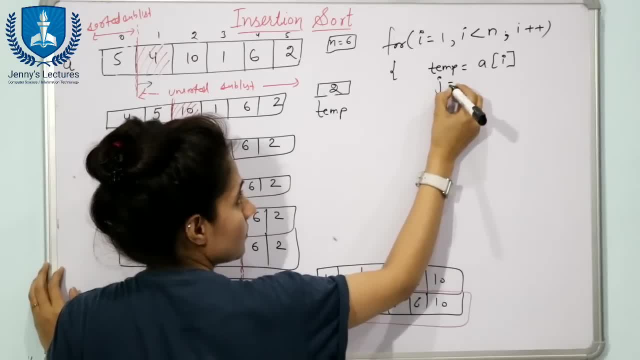 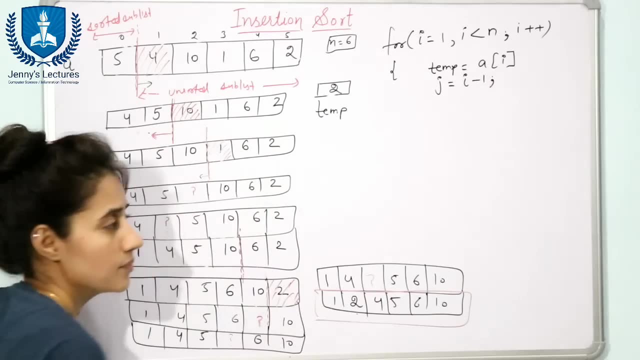 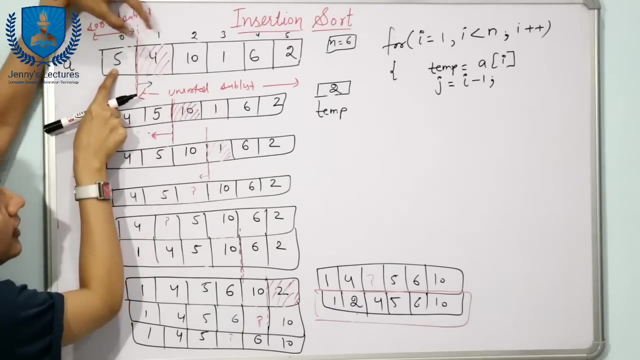 be decremented. so let us take one variable, j, fine, and we take this. we initialize this variable from first loop, that is j, and then we take: j is equal to i minus one. why so? because, see, when i is one, then we have compared this four with the five and the index for this is zero. that is why i am taking. 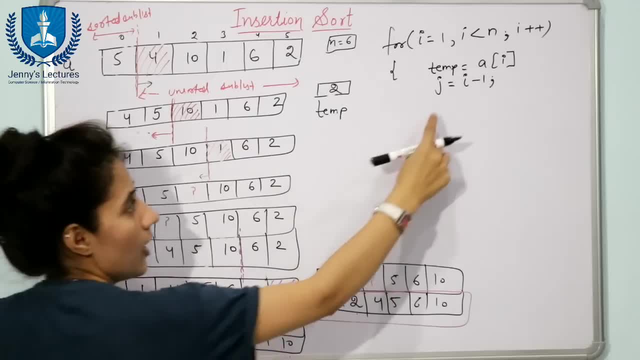 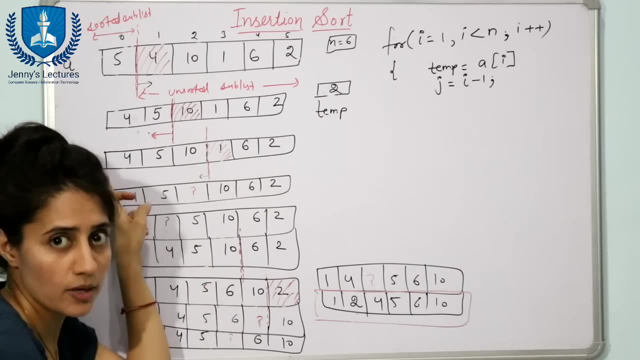 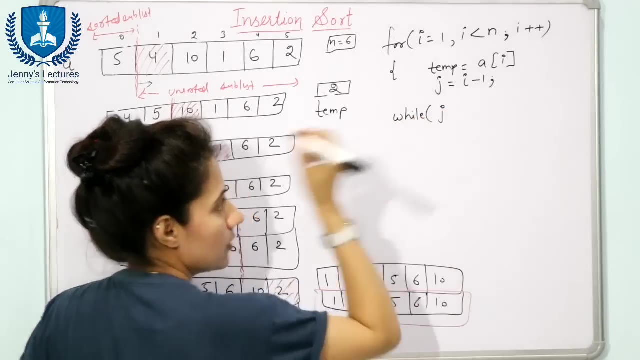 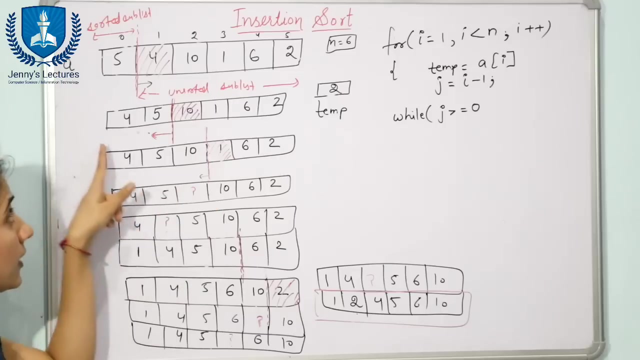 j is equal to i minus one. so here i is one and j is zero. now we will start the loop for this j. for the loop for the comparison, we have compared all this value with temp variable till we reach to zero. now we'll start the loop while j is greater than or equal to zero, greater than or equal to index zero. so 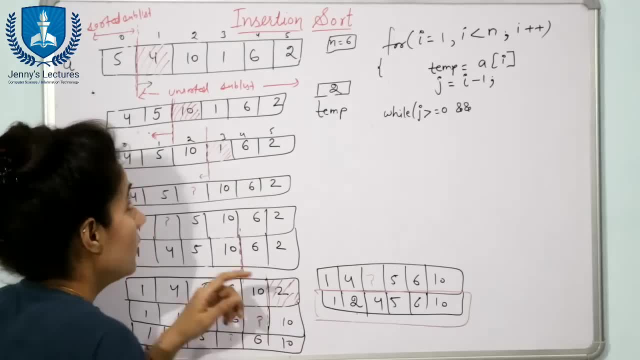 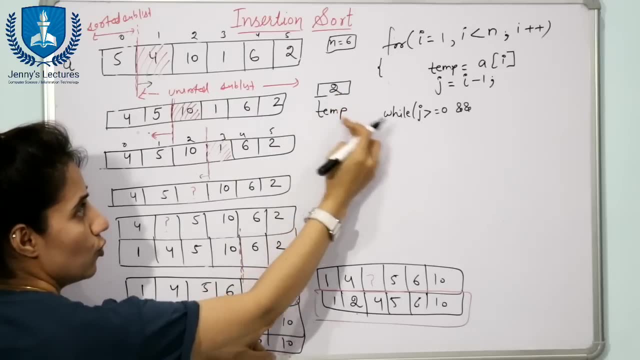 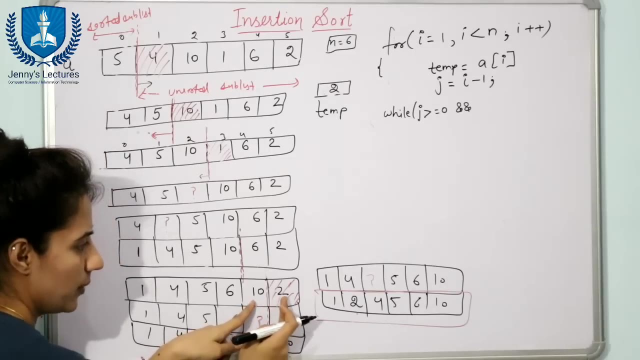 first condition is this: and and next, what we have done, we have compared, we have compared, see, suppose we have taken this here. in this case, we have taken two and we have stored two in temp variable right now. we have started, we have started, we have, we have compared this two with. first to 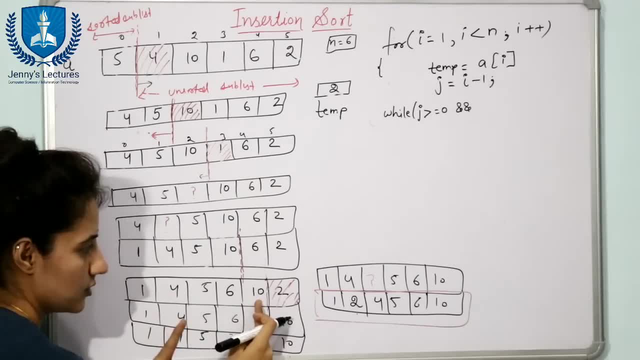 say that so this value is zero, this value is five, and then times ten, then five, this four, and then so i combined this we have into one decimal, and then times five, and then six, and oh, this 10. okay, we had done all this. ten, then six, then five, then four, and then 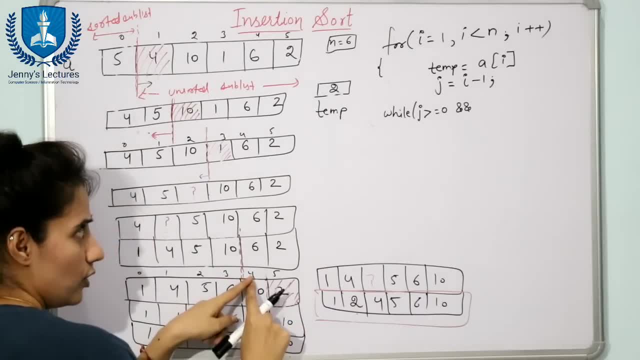 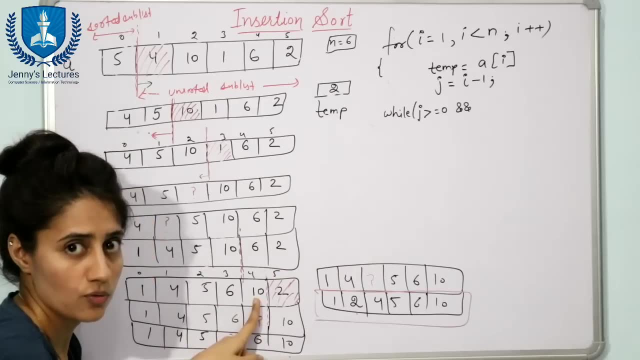 one like this. fine, now we have started from here only. fine. so j value is i values index is 0, 1, 2, 3, 4, 5. so here i value is 5, j value is i minus one, that is four. fine, now check, j is greater than equal to zero and this value, this value, 10, is greater than temp value. happiness value is greater than loves volume. so how to write this one? A, O equal to 0, like ethi is greater than or equal to 0. so let's say we're 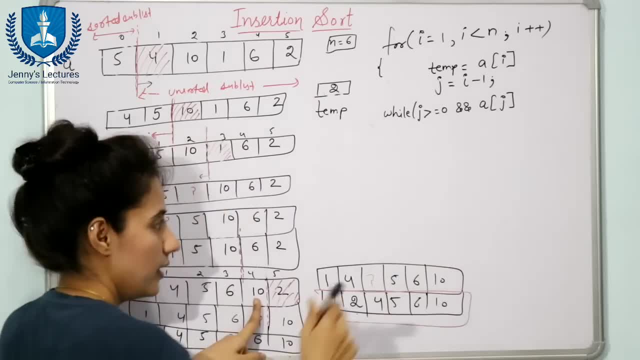 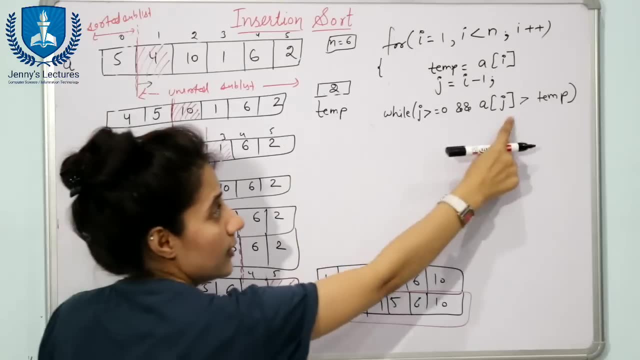 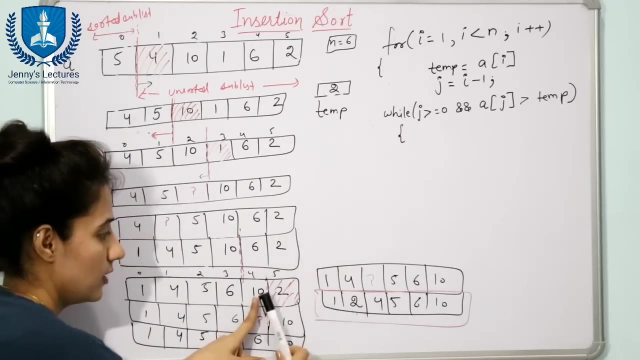 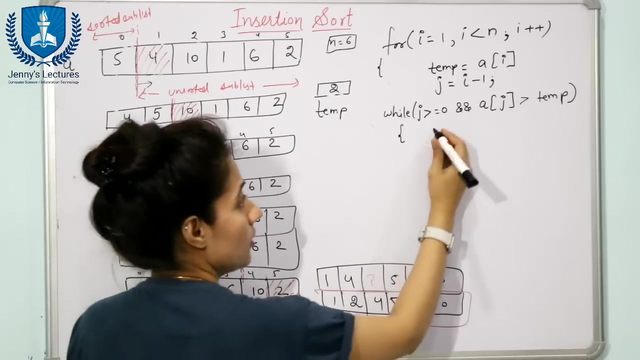 of j greater than so. this a of j, a of j greater than 10. if both condition are true, then what you will do. if this was greater than see, this 10 is greater than 2, then we have, we have shifted this 10 one place, right. fine, now how to write this one. 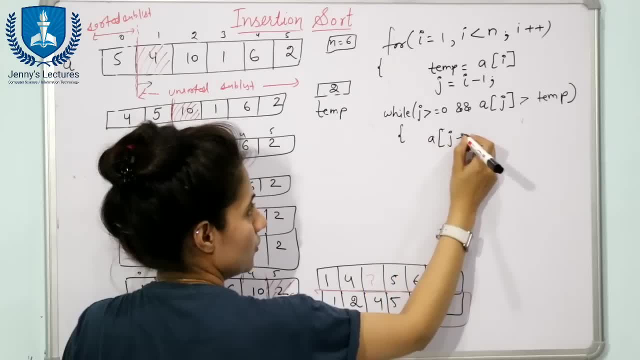 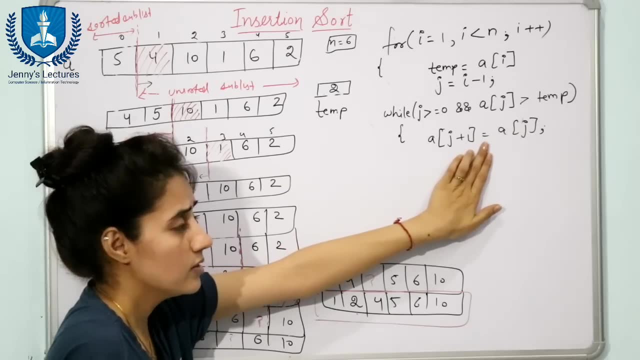 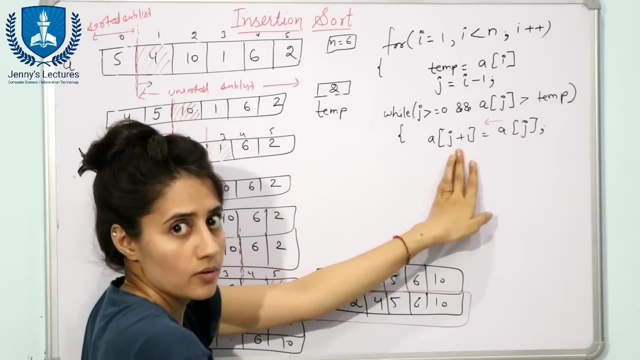 so a of j plus 1 is equal to a of j. fine, when you are going to write this, equal to operator, it means the right value. the right value is to be assigned to the left variable. this is the here. only. fine, so this value, a of j, would be assigned to a of j plus 1. obviously we have. we. 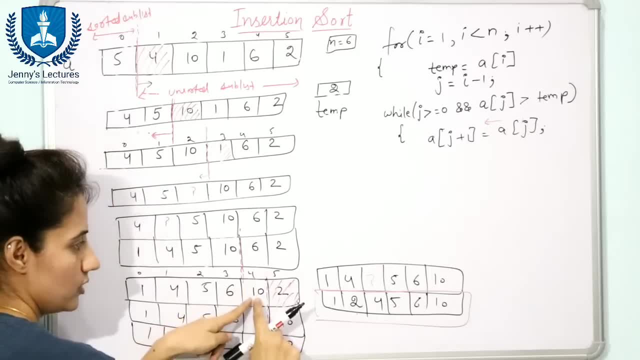 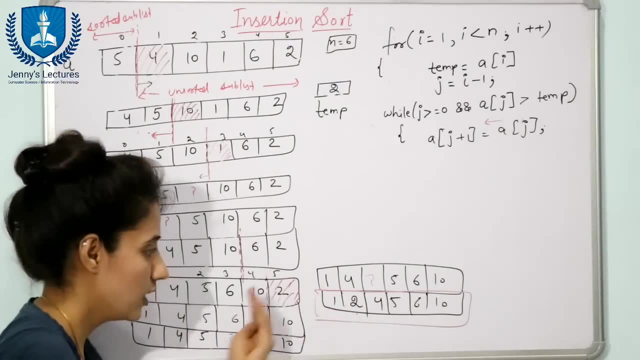 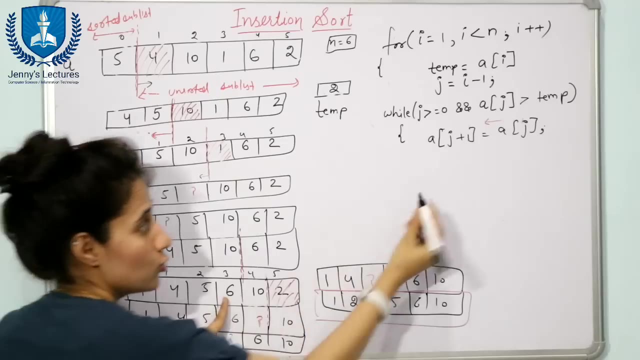 have right shifted this 10, so a of this 10 was first of all in a of 4, you, and after that we have put this 10 a of 5, fine, so at j plus 1 value, and then again we compared with this 6. it means j value is has been decremented by 1, so here you will write what j. 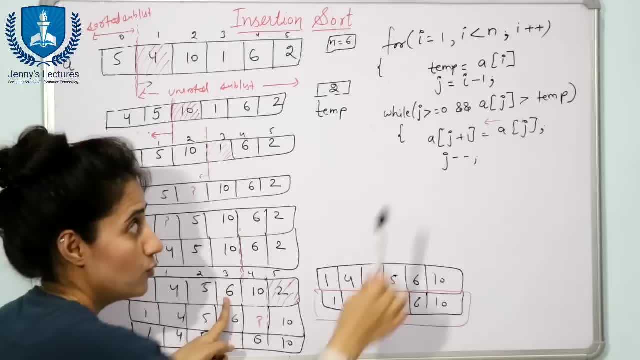 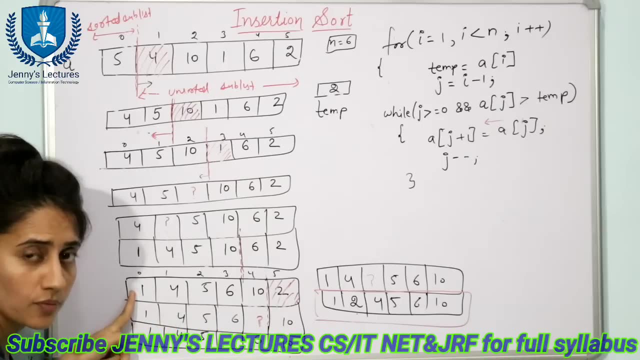 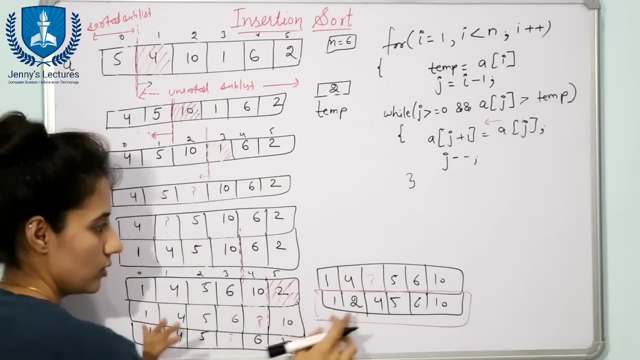 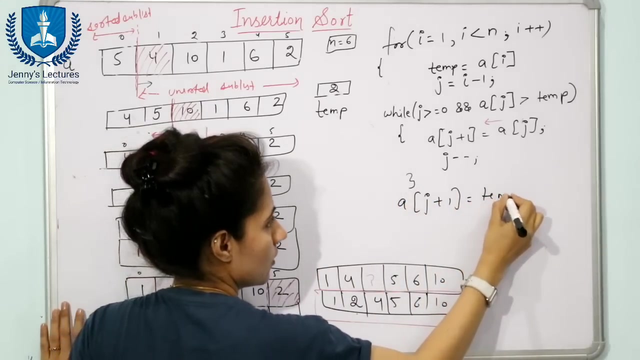 minus, minus, fine. if both conditions are true, then this loop would be going to 0, to index 0, fine, and after that. after that you will here, you will store what, here now we have stored what, this key value, sorry, the temp value, so where you will store a of j plus 1 is equal to 10, so this is the while loop. 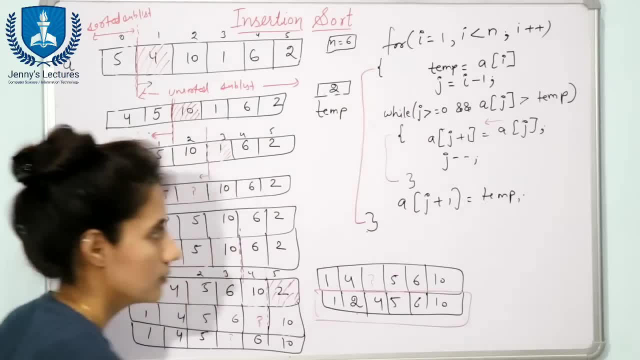 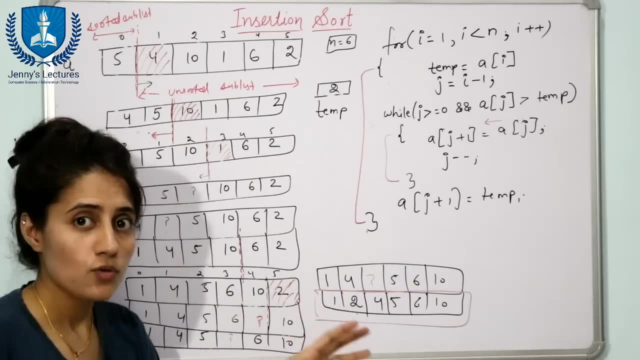 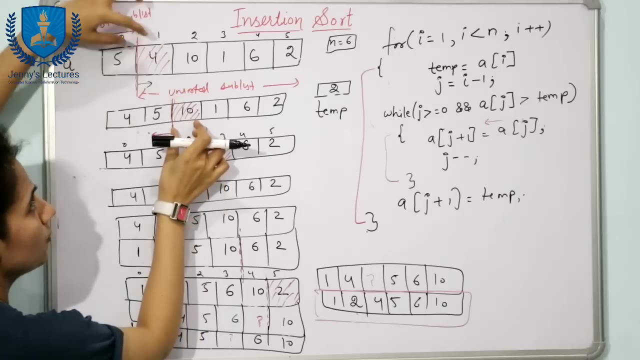 and this is the outer for loop. fine, a of j plus 1 in. in a of j plus 1 you will store what temp. now let us take one example and trace out this code. see, let us suppose we are going to take this 10. now, fine, we have taken. suppose we are not going. 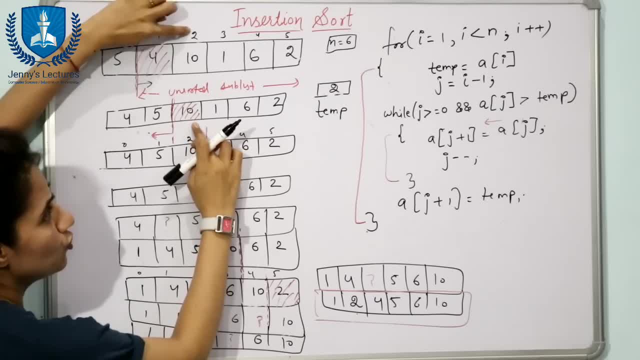 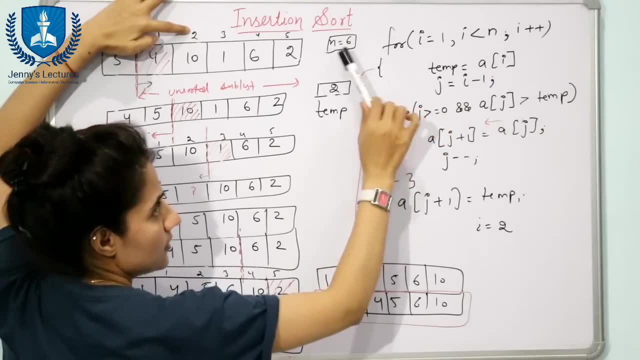 to take 4. we are going to take this 10. i value for 10 is 2. now suppose i value is 2. fine, i is 2. 2 is less than n. 6. yes, condition is true. then we are going to enter in this in temp. 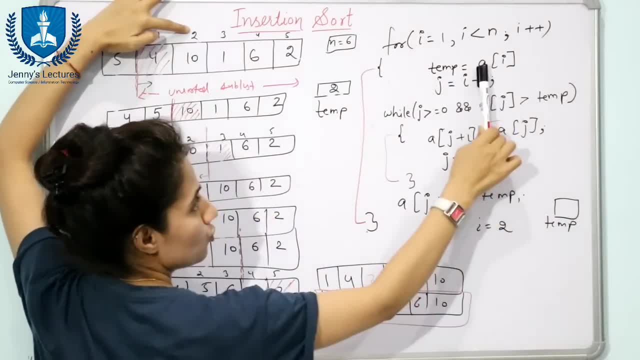 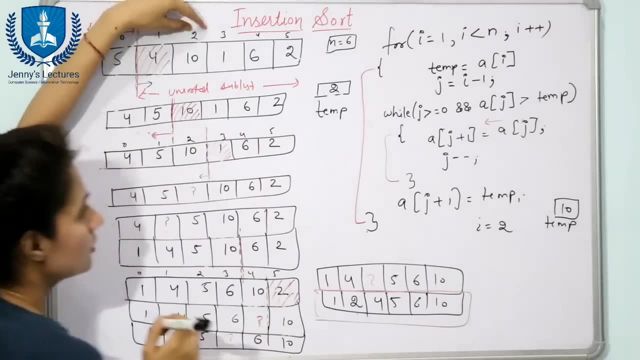 in temp variable. we are going to store a of i, a of 2. now. a of 2 is what a is name of array, a of 2 is what n. again in temp, we are going to store this 10, fine, and this is considered as a whole. now, now. 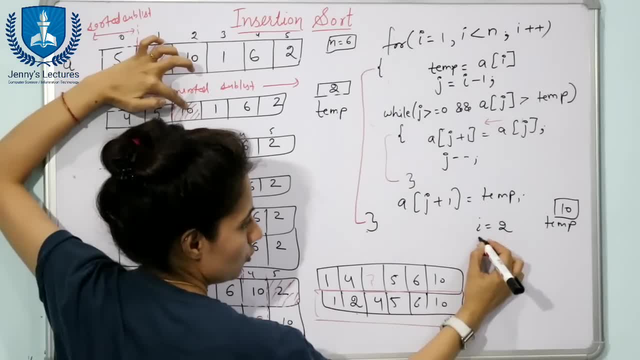 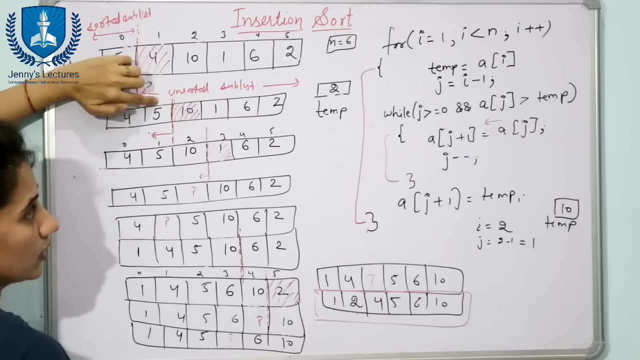 now see: now j is equal to i minus 1. now j value is what? 2 minus 1, that is 1. now j is equal to 1, index 1. we are going to start from here. only now check: while j is greater than equal to 0. 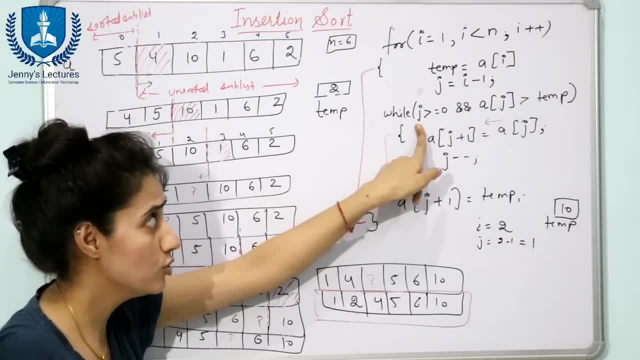 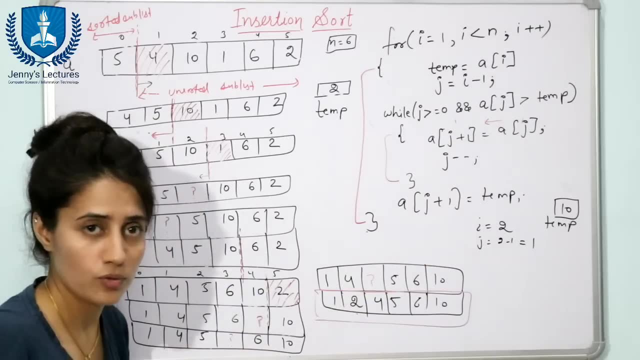 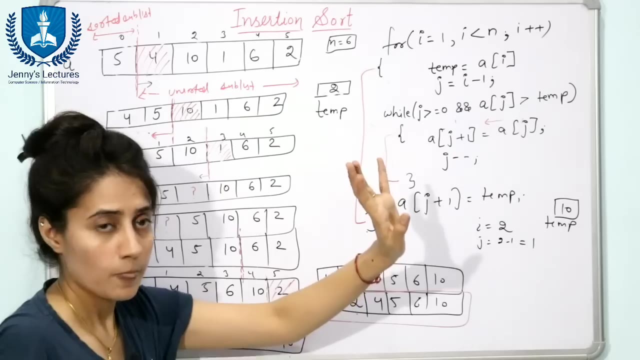 j value is 1. yes, this condition is true. fine, one condition is true. hey, this is logical. and for entering this loop, these both conditions have to be true. if this condition or this condition, either one condition, is false, then control will not enter in this loop. now, in this case, this condition is true now. second, 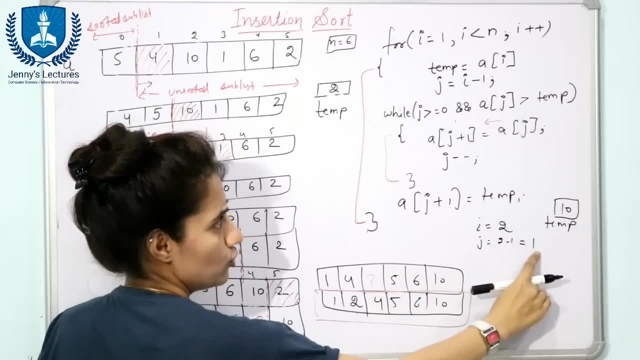 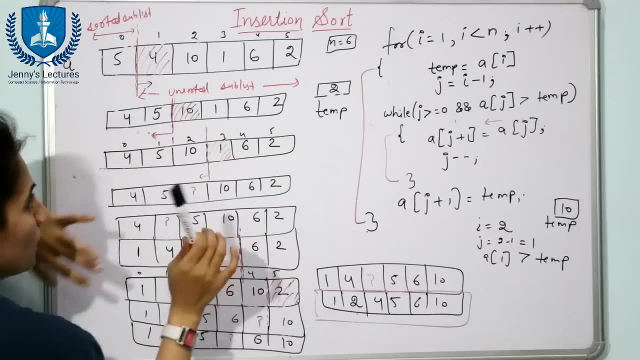 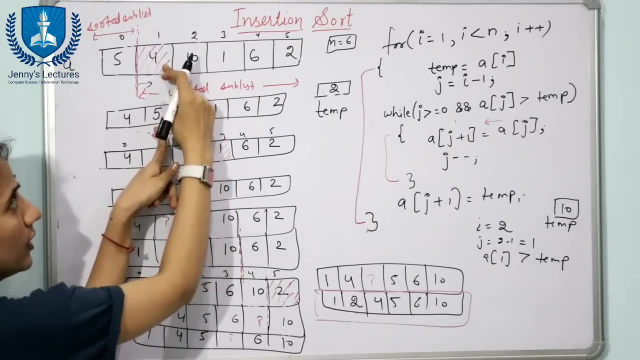 condition is a of j. j value is 1, so a of 1 greater than 10. so now here, a of 1 is what? here, a of 1 is 5. fine, see, we are not going to take this 4 here, because after inserting 4 at this proper place, 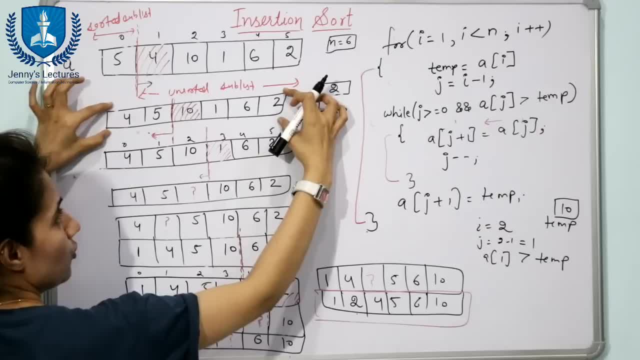 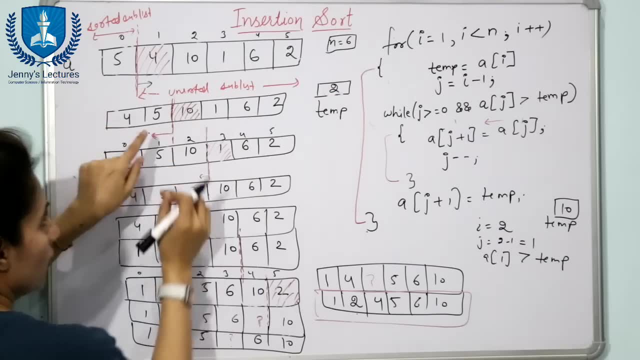 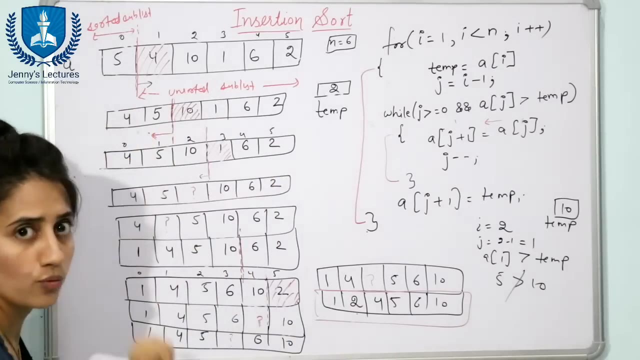 now. array is now our array is this one. when i value is 2, at that time array is this one. so we are not going to consider this array. we are going to consider this array now here: a of 1 is what 5, 5, 5 is greater than 10. no, this condition is not true, so we will not enter into this loop. 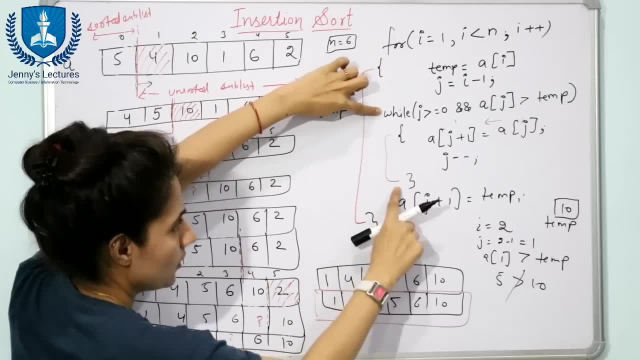 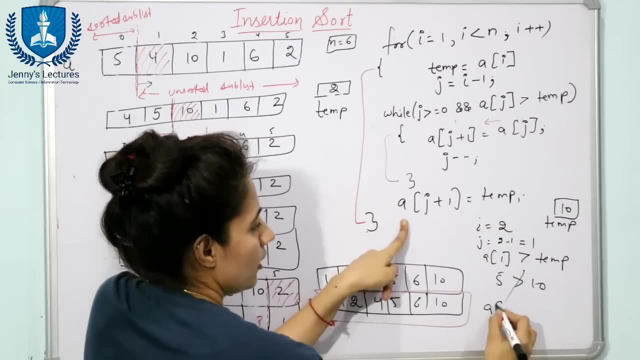 fine, if you will not enter into this loop, then from out of this loop the statement is: a of j plus 1 is equal to temp. now a of j, j value is 1, 1 plus 1. a of 2 is equal to temp, value is 10.. 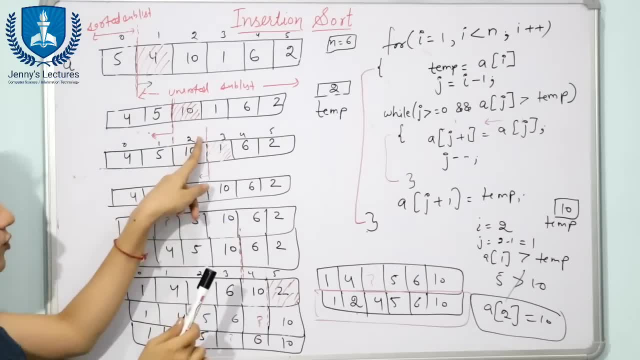 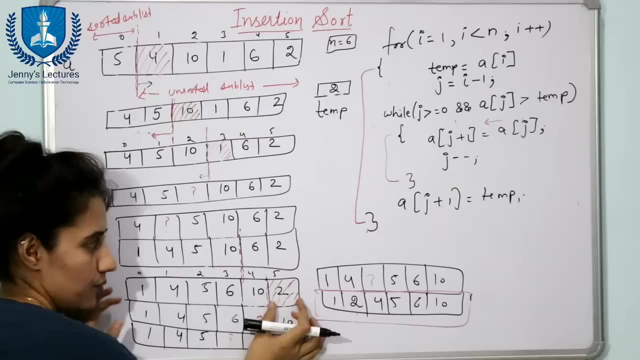 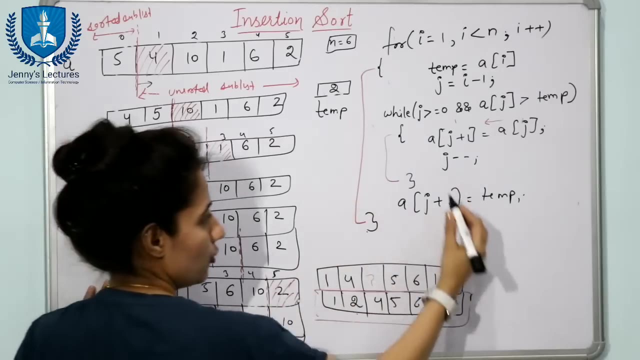 now, in a of 2 you will store 10, and obviously in a of 2 we have stored 10.. now let us take another case. suppose we are going to take this value 2, fine, and here, if we are going to take this 2 value, then here i value is what 5.. so now suppose i am going to 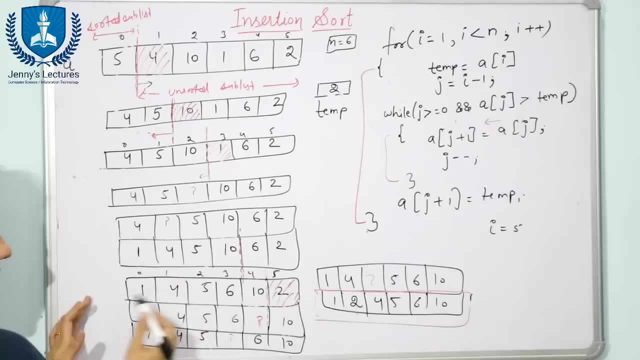 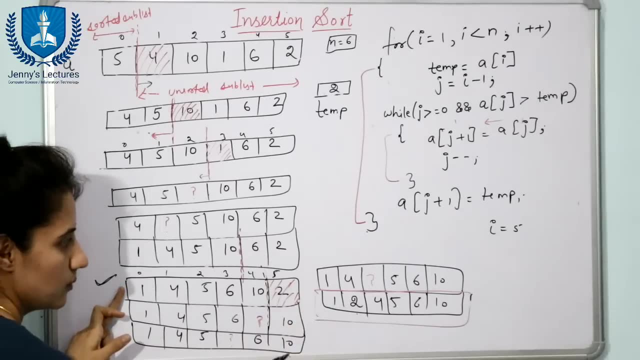 take a case where i value is 5. so in that case, array is this one. we are going to consider this array now, because this is sorted array and only this. this 2 is an unsorted list. 5 is less than 6. yes, condition is true. we will enter in this loop now in temp. you are going to 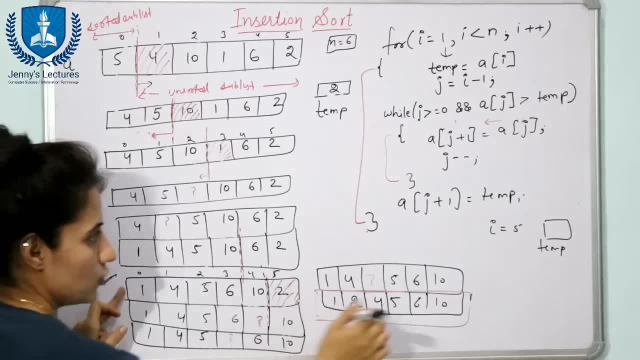 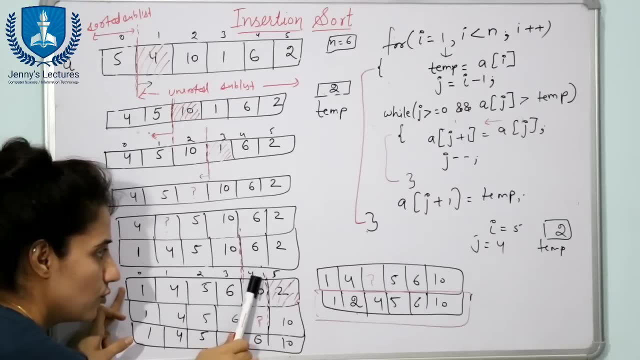 store a of i, a of 5. a of 5 is 2. we are going to store 2 here now. j value is i minus 1. j value is 4.. the loop would be started from a of 4 here, 4. fine, now check. this condition is true. j is greater than. 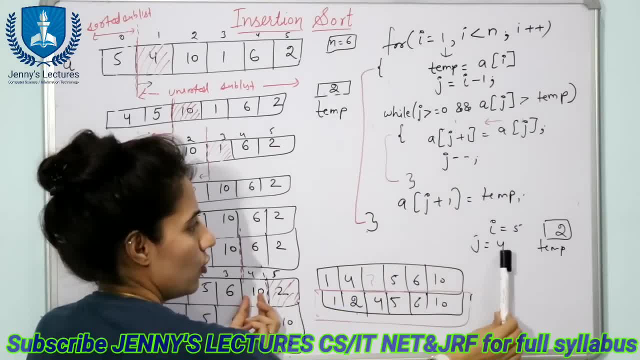 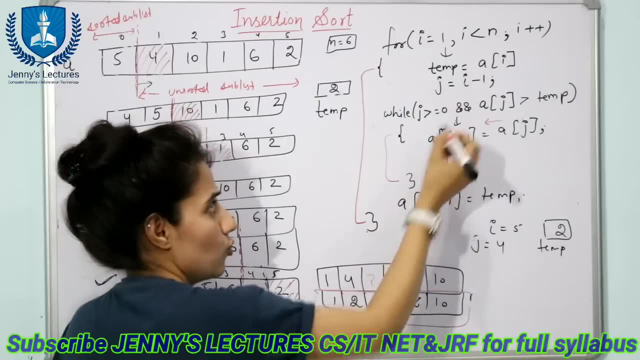 0. yes, 4 is greater than 0. true, and a of j. a of 4. a of 4 is 10.. 10 is greater than this temp value. yes, both conditions are true. then we will enter in this loop. then what will happen? a of j plus 1: see. 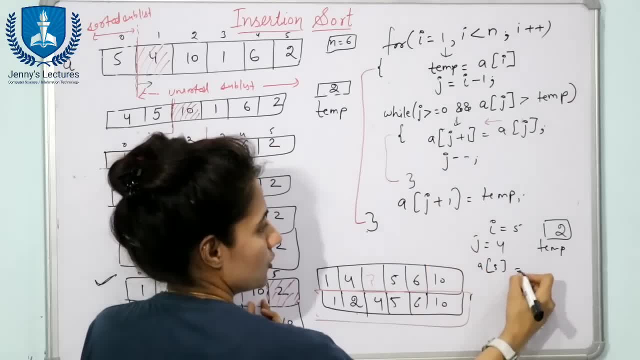 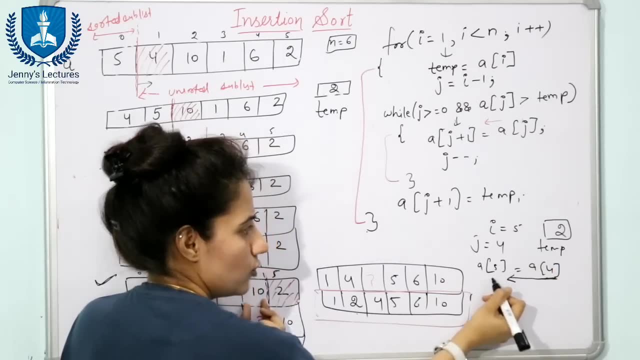 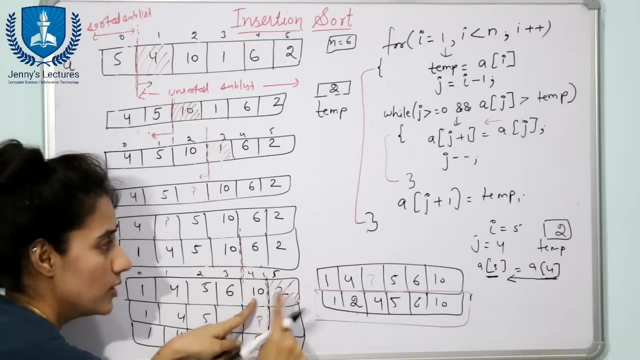 j plus 1 means 5. 4 plus 1. 5 is equal to a of j a of 4.. it means the value of a of 4 would be transferred to a a of 5.. now value of a of 4 is 10. this 10 has been transferred to. 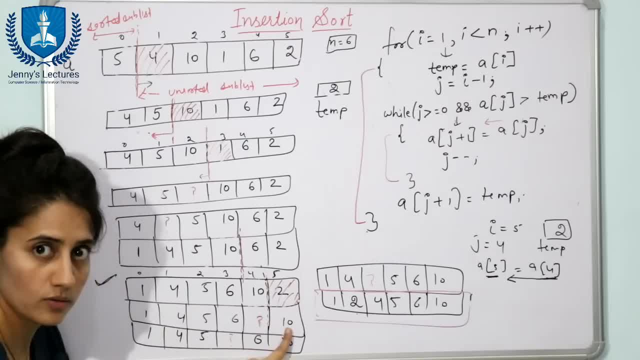 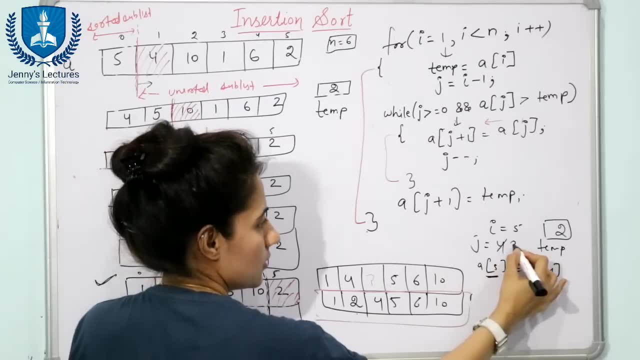 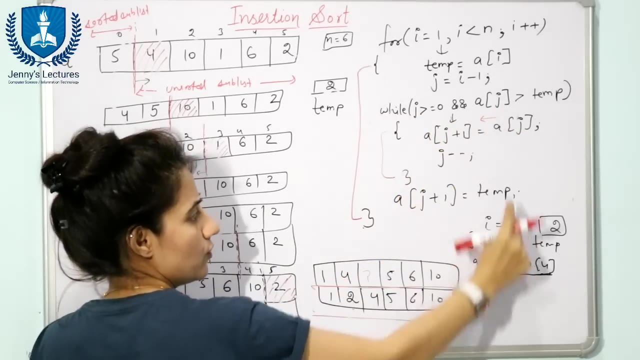 will be transferred to a of 5. here only, we have done. fine, this is a of 5 done. now. next step is j minus 1, j minus minus. so now j is 3. fine, now check again: 3 greater than the 3 is greater than equal to 0. yes, and a of j means a of 3. 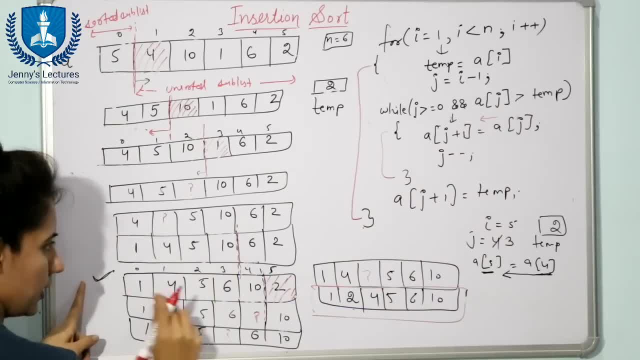 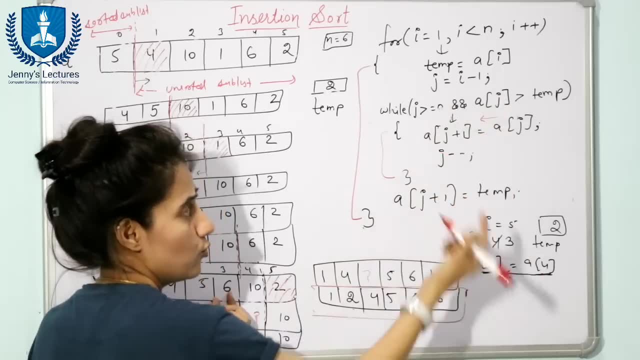 what is a of 3, a of 3? a is this name of this array index? is 3 a of 3? is what 6? 6 is greater than 10? 6 is greater than 2? yes, both conditions are true. we again enter it in into in this loop. 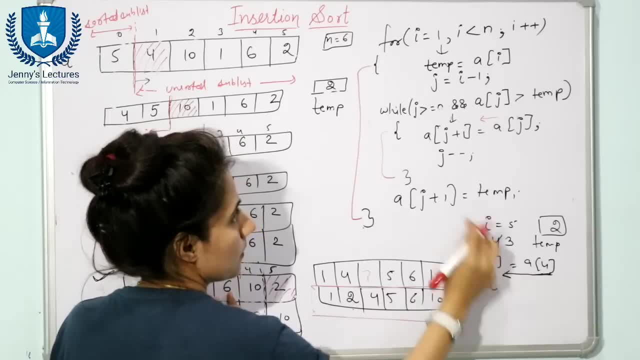 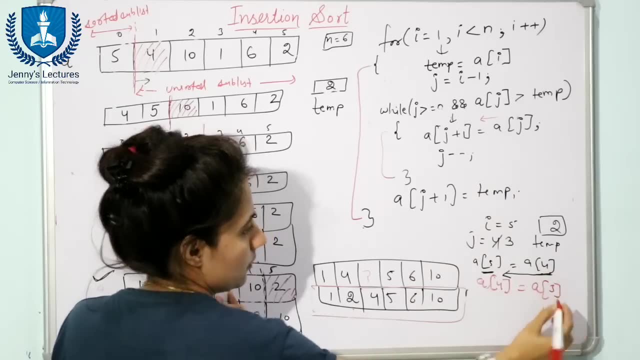 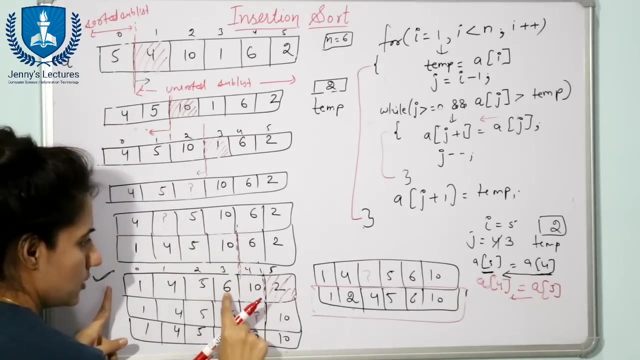 and what will happen now? a of j plus 1 j is 3. a of 4 is equal to a of j is 3. it means the value in a of 3 would be transferred to a of 4. now what is value in a of 3? a of 3 is 6. 6 would be. 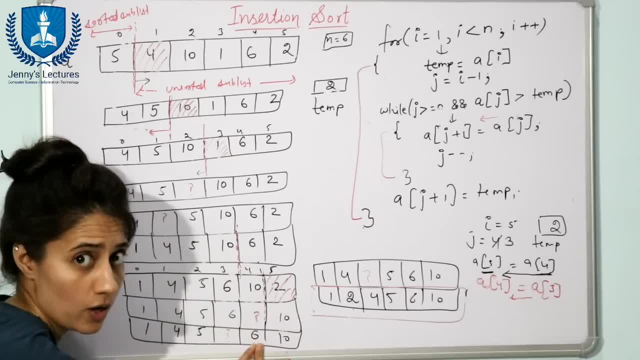 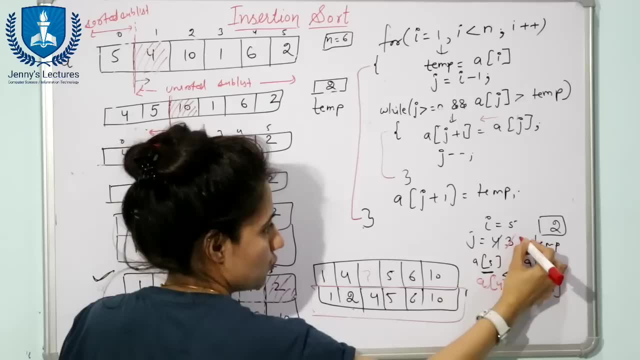 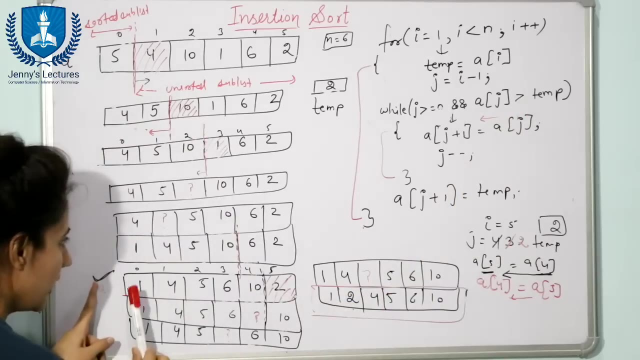 transferred to here only a of 4, as we have done in when we are discussing this numerical. fine, now this has been transferred. now j minus minus. now j is what 2? now again, 2 greater than equal to 0. yes, a of 2 greater than temp. what is a of 2? a of 2 is what 5? 5 is greater than temp. yes. 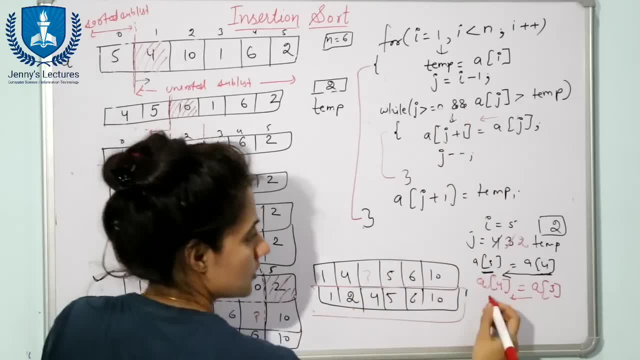 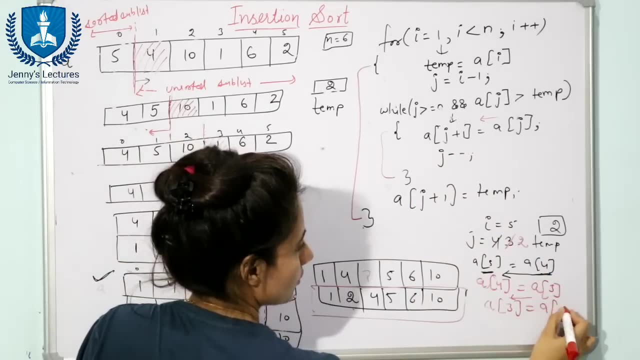 both conditions are true, again, we will enter it in into this loop. and what will happen now? enter in this loop. what is the first statement in this loop now? a of j plus 1, j is now 2. 2 plus 1 is 3- is equal to a of j. it means the value in a of 2 would be transferred to a of 3. what is? 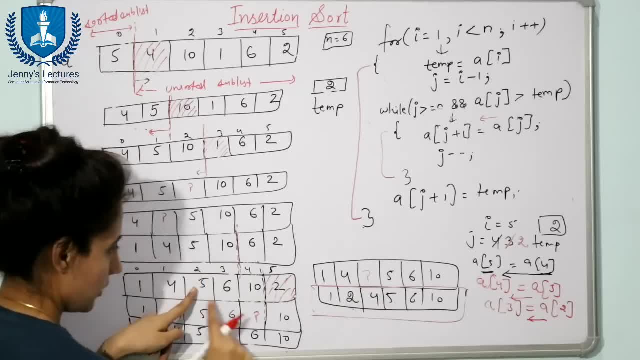 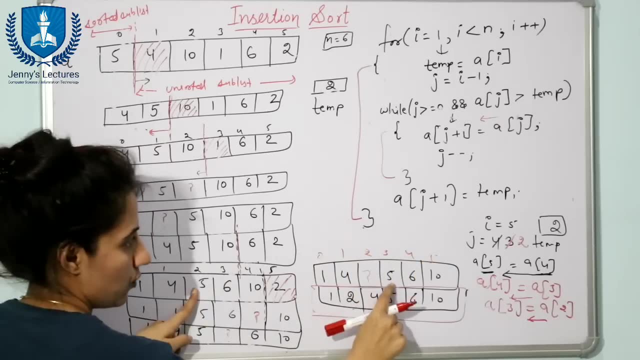 value in a of 2, 5, 5 would be transferred to a of 3. see, we have transferred here only index 0, 1, 2, 3, 4, 5, 2, now 5 is a of at a of 3. fine, j minus minus. now j is what. 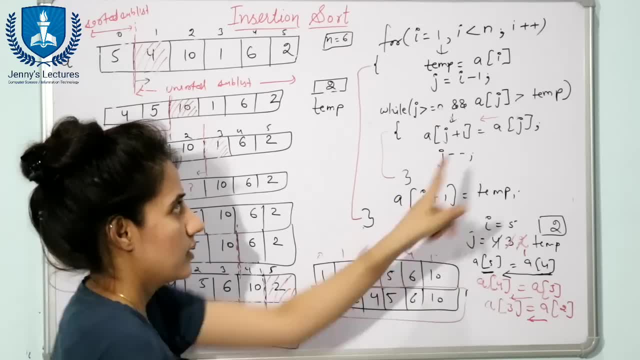 1, 2, 3, 4, 5. now 5 is a of at a of 3. fine, j minus minus, now j is what 1, 2, 3, 4, 5 is equal to a of 3. 1, now 1 is greater than equal to 0. yes, and a of 1. a of 1 is what a of 1 is what 4, 4 is greater than. 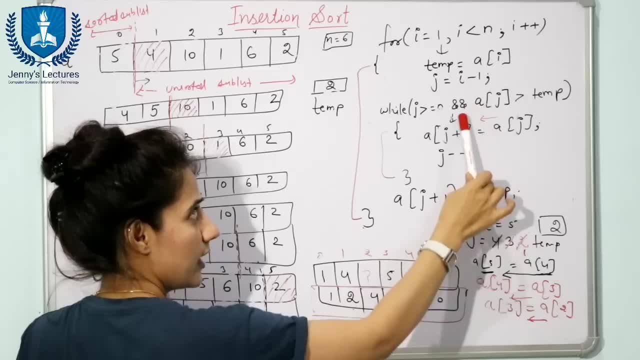 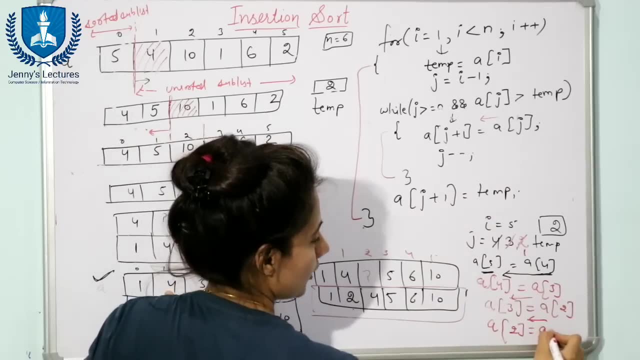 temp. yes, this condition is also true. both conditions are true. we will again enter in this loop now. statement is: a of j plus 1. j is 1, 1 plus 1. a of 2 is equal to a of j. j is what 1 it means. 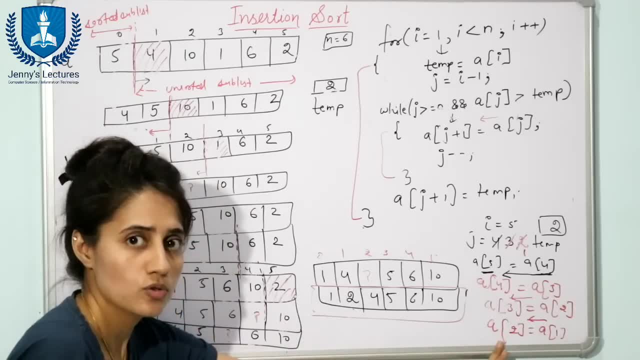 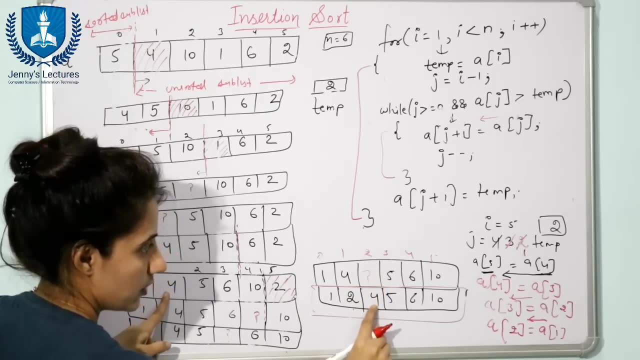 a of 1 value would be transferred to a of 2. now, what is a of 1? a of 1 is 4. this 4 would be transferred to a of 2, see index is 2. here we have 4 now. fine, now. next is j minus minus. now j is what? 0? fine. 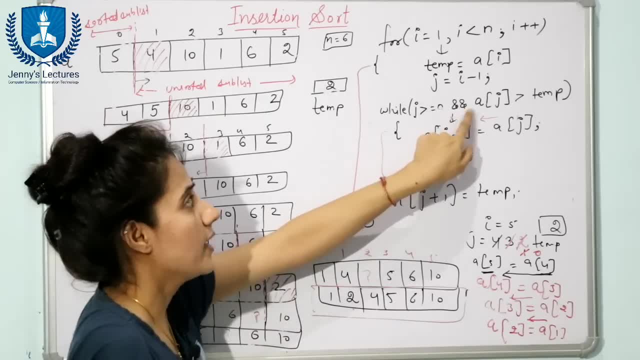 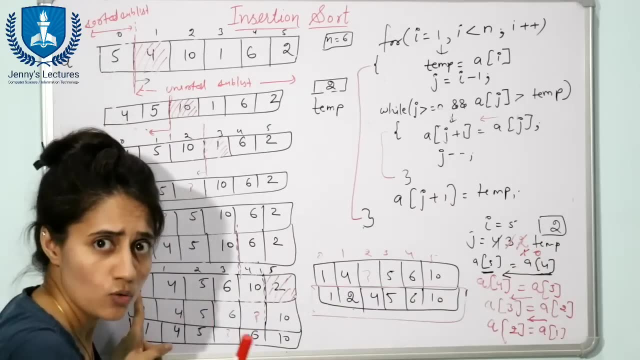 0 greater than equal to 0. yes, this condition is true. and a of j, a of 0 greater than temp. now, a of 0 is 1 and temp value is 2. 1 is greater than 2. no, this condition is not true, only this condition is. 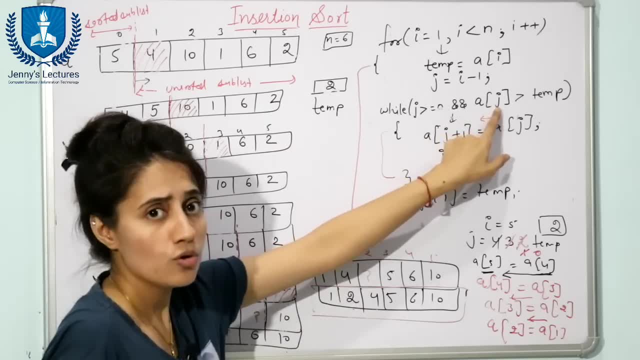 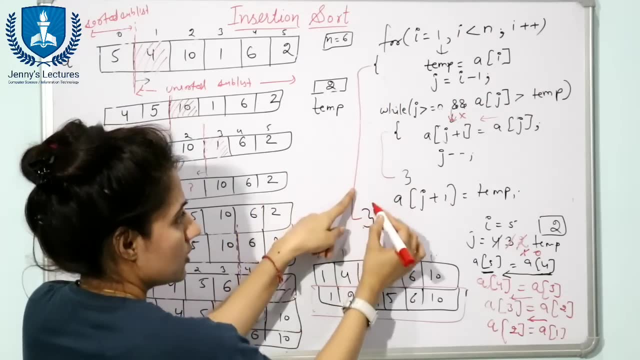 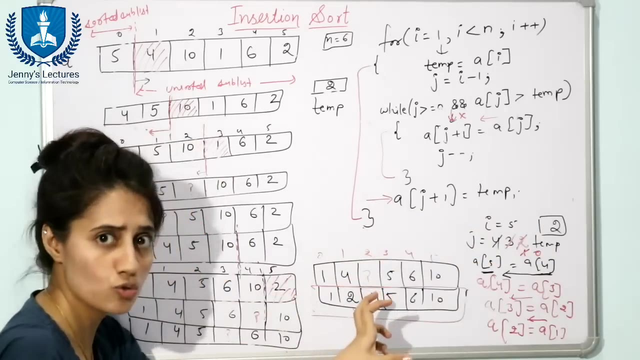 true. this condition is not true. if one condition is not true, then we will not enter in this loop. control will not enter in this loop. fine, now, after this loop, whatever is written, the control will go to that statement. now, here, what is written? a of j plus 1 is equal to temp. now this temp value has been stored. we have find. 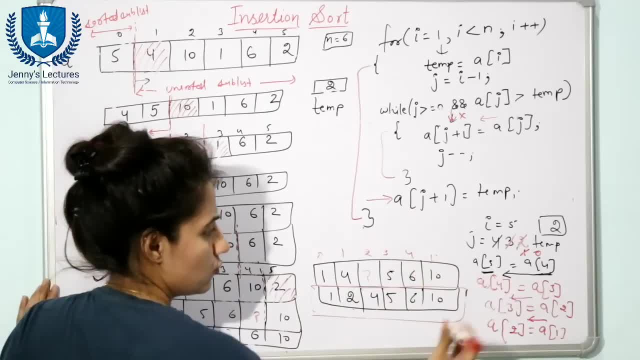 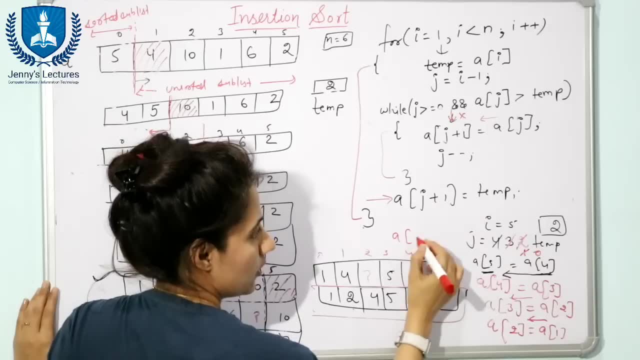 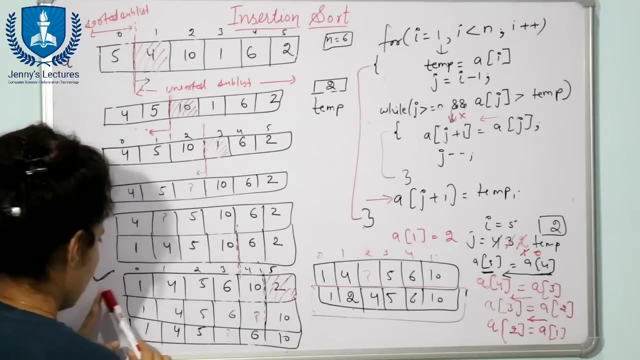 out the appropriate place now. a of j plus 1 is what see. a of j is what 0 in this pass. so a of 0 plus 1 is a of 1 is equal to temp. temp is 2. now now, what is a of 1? see a of a of. 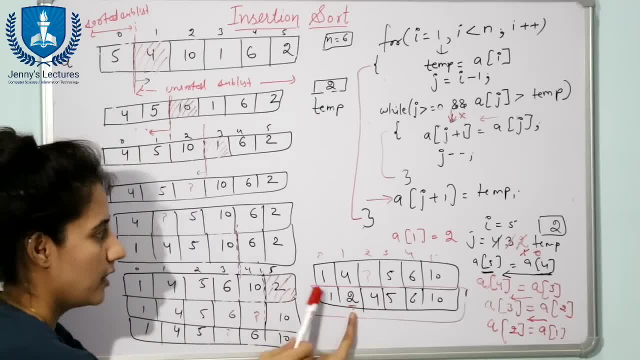 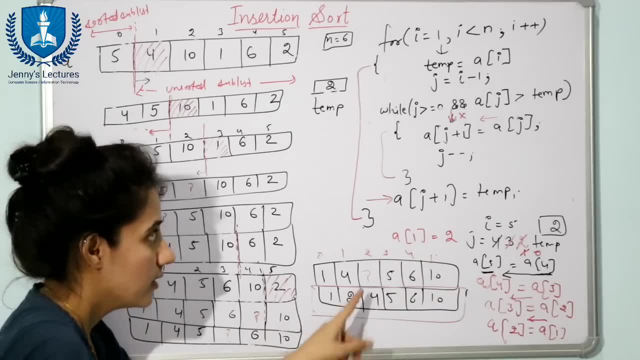 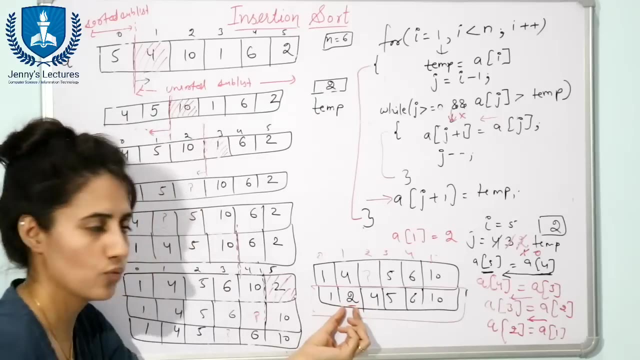 1. here we have stored 2. at a of 1 index is 1, same we have done when we are discussing this numerical and when we are trace out this, this code. then also you find out that at a of 1 only you are going to store this 2. it means this code is right. so now the time, complexity, both in worst. 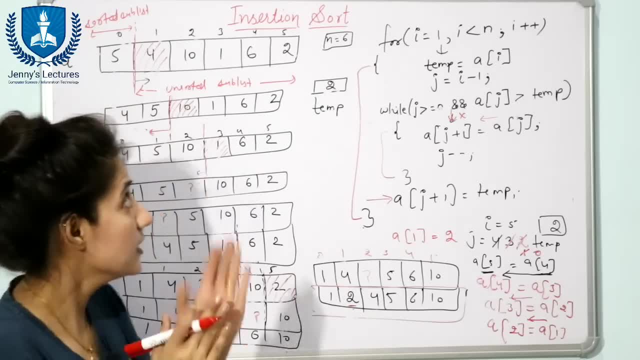 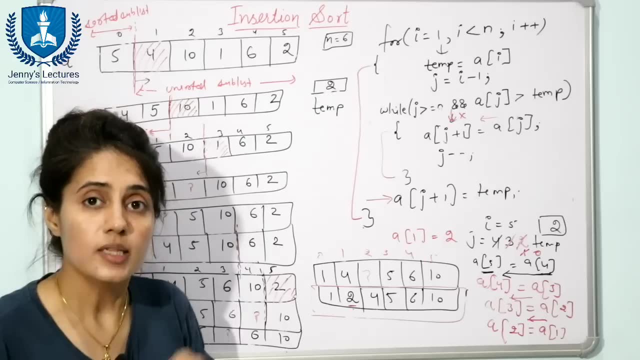 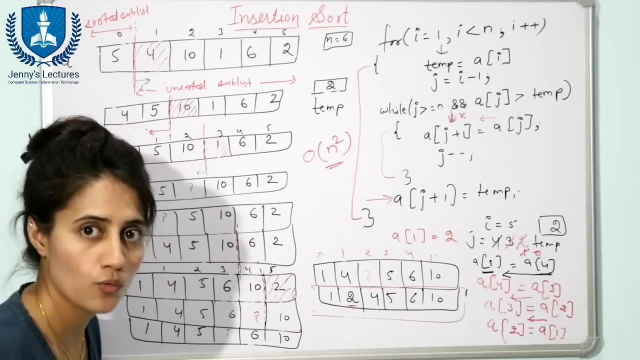 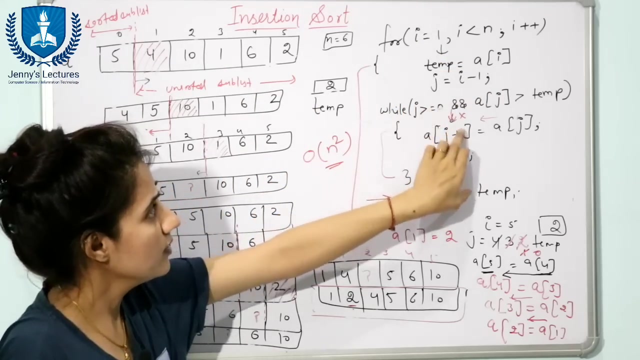 case and best case. now see, the worst case is what? when the array is given in descending order and you are, you are going to sort the array in ascending order. that is the worst case. in that case, time complexity of this sort is order of n- square. why so? because, see, this loop will also go from 1 to n. fine, and and within this loop, 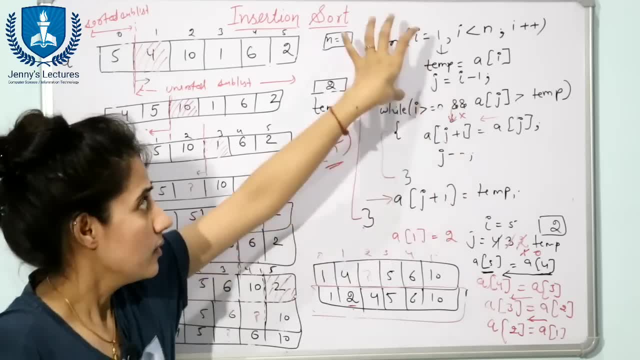 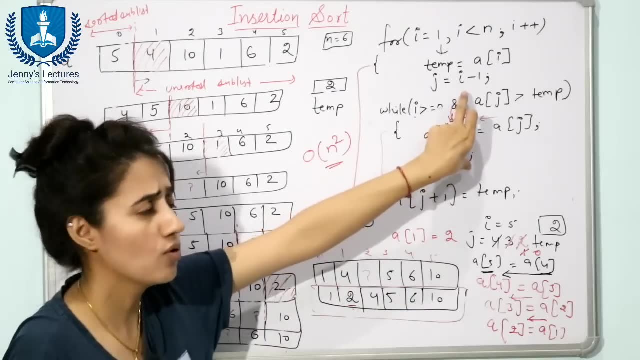 one while loop is there. okay, now when loop nested loops are there, then to find out the time complexity, you just calculate the number of computations of the inner loop and after that you can find out the time complexity. now also, the inner loop would be started from i minus 1. 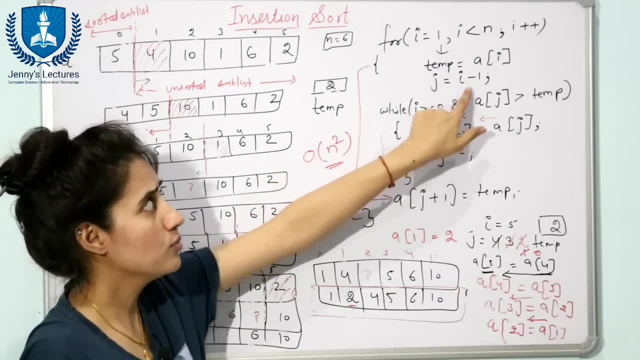 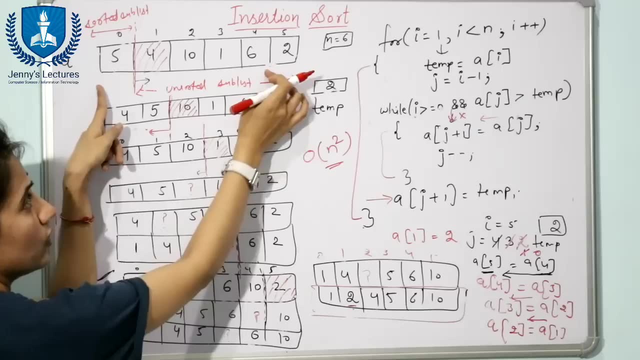 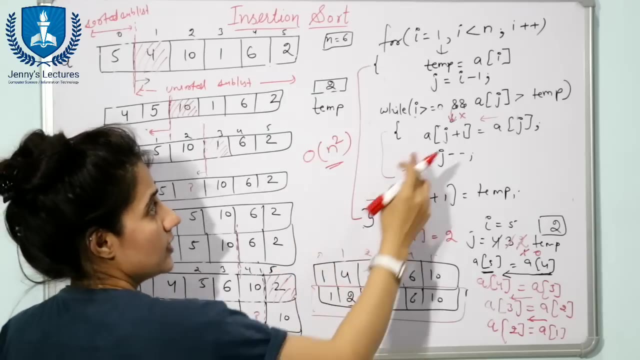 fine. if i value is 1, then from 0. if i value is sometimes 5, okay, then j would be started from 4. we are going to compare this value with all the variables in the sorted list. when the worst case is there, fine. so in that case the time complexity would be n square. this loop is also going to be. 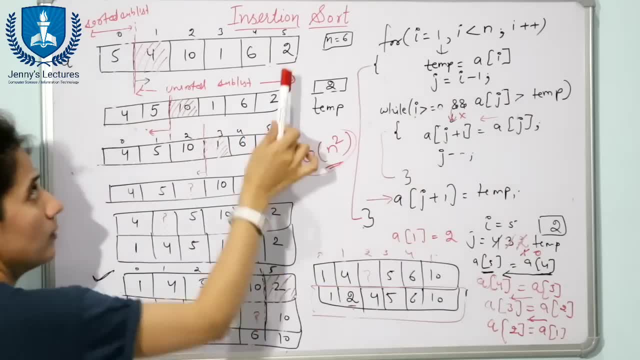 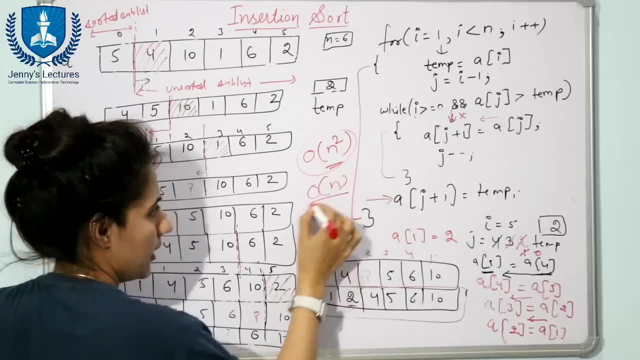 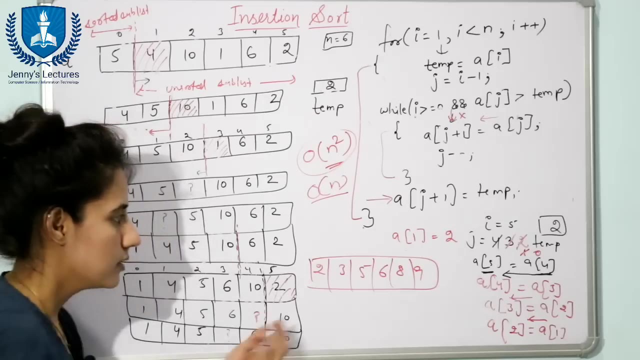 from one to n, and this, this will also going from here to here, only in the best case. time, complex, time, complexity is order of n. why so? best case is what? the array is already in ascending order. okay, like this, this is the array given. this is the in the ascending order. fine, starting this. 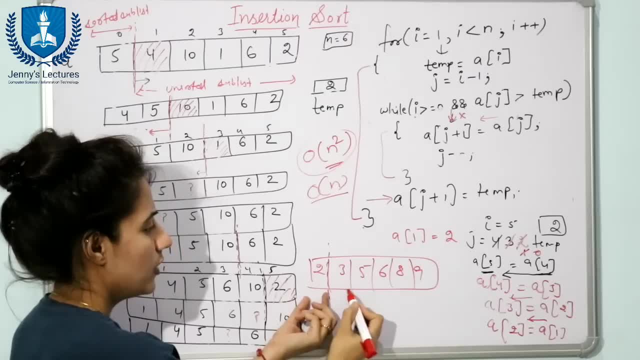 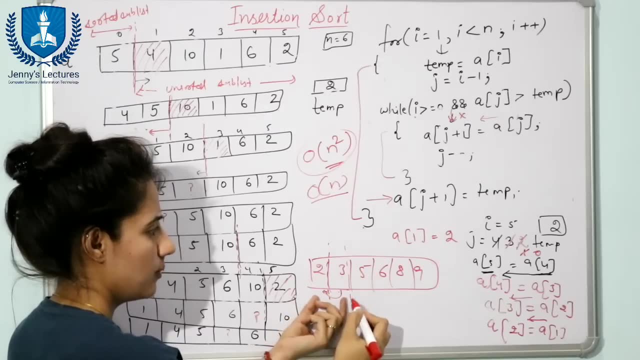 is the sorted sub-list in starting, and this is unsorted sub-list. we are going to take this three. we are going to compare with two, not less than three. so three would be inserted here only now. this is the sorted sub list. now we are going to take five. we are going to compare this five with this three only. but this three is.